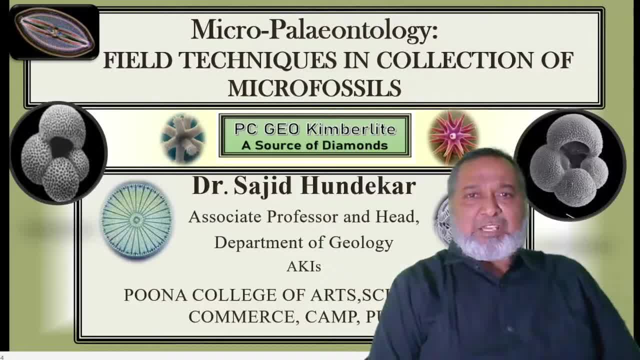 in collection of microfossils. I am Dr Sajid Undekar, Australian professor and head Department of Geology. aka is Pune College of Arts, Science and Commerce, Camp Pune, Maharashtra, India. So micropediatology Now. for this we require, a special technique is required. 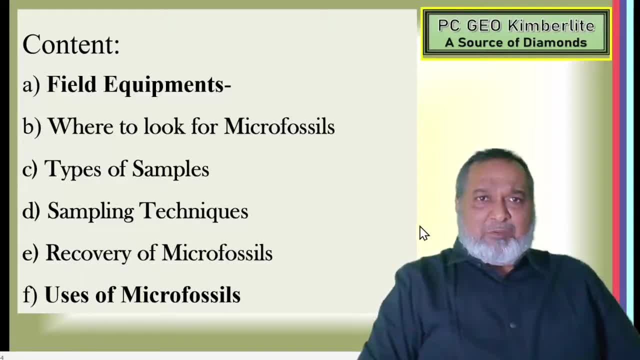 So in this topic, this topic, we will divide it into field equipments where to look for microfossils, types of samples, sampling techniques, recovery of fossils. If it is possible, we will make a in this. otherwise, 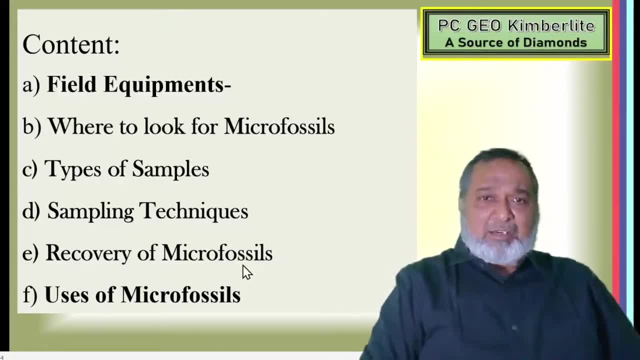 if it is become big one, then we will make the recovery of fossil as a separate topic. Then uses of fossil I made as a separate because I feel this topic will become a very big one. So uses of fossil, already uploaded on my channel, PC Joe Kimberley, and that is a short video, is 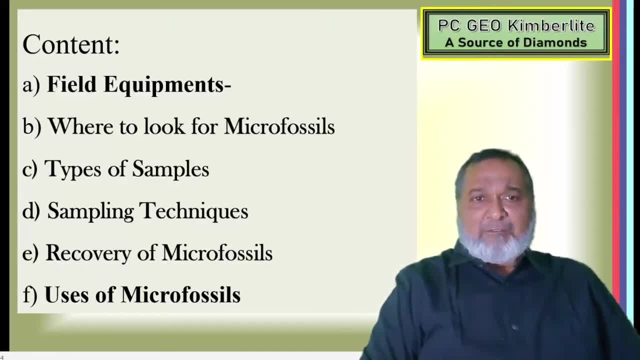 there, So you can watch it, So you can enjoy that. uses of fossil. So here field equipment where to look for fossil microfossils, type of samples, sampling techniques and if possible we will take a recovery of microfossils. 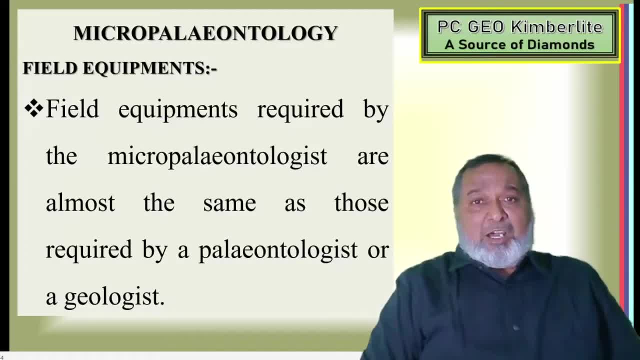 Yes, Field equipment: What are the field equipment required for the micropediatologist? That is a very, very important. Whenever a micropediatologist is planning to go for uh field work, he has to have the first one: the what topic? what exactly the fossil he wants to looking for? 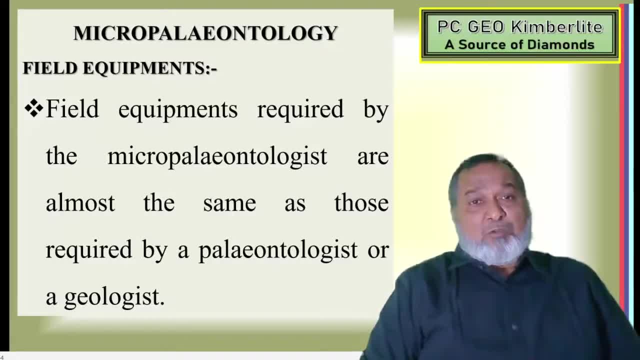 whether you want a foraminifera ostracot conodon, what will be the age? and once you make out, then he has to make. go on, refer the various research papers in which particular area we are going to get this particular micro fossils on the. 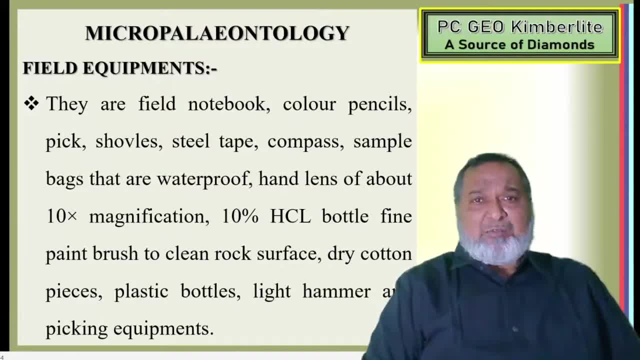 field. We can make out that and with this we have to start, uh um, getting the research material. then the next one, very important. Once he has got this one, then the next very important one to push it map of that area where he is going for that. 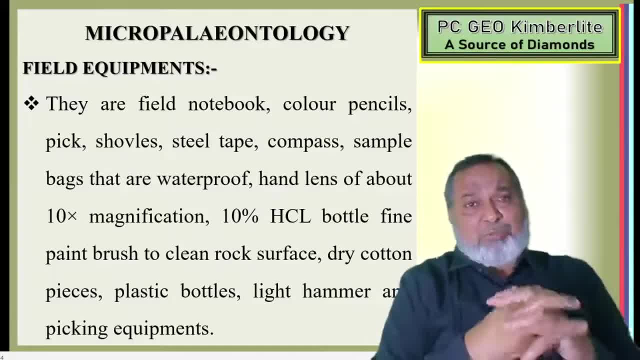 And, uh, after the completing these two important things, keeping in the mind, uh, how many days he has to plan for the microfossils collection? Uh, two is there, whether it is seven days, four days, whether it is two weeks, plan planning is there? 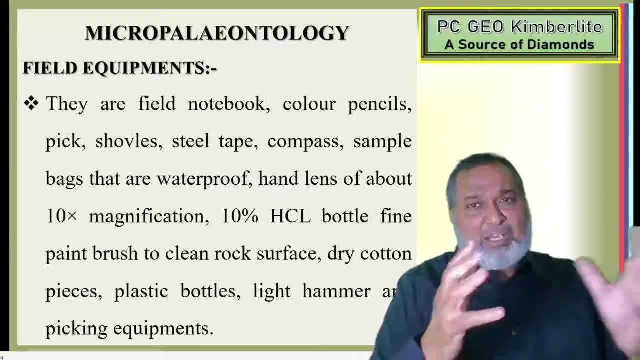 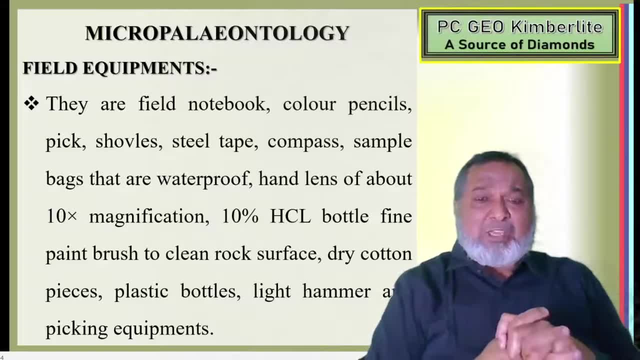 So he has to properly plan then accordingly, the rest of the thing he has to start making note downing the things that these are the requirements, will be there for the field work. The first foremost field notebook, this will be required, the field notebook, because wherever he is taking the observation, reading is taken. 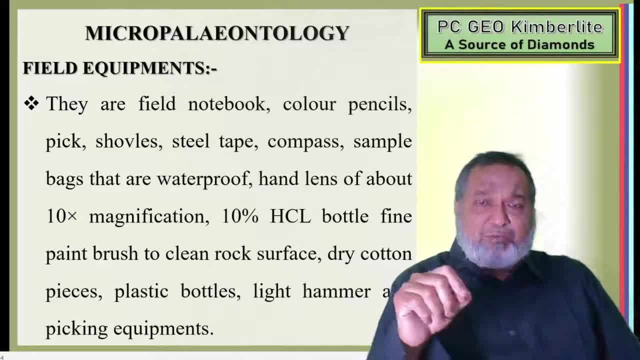 Now note down in the field. what are the characters of the rock which are exposed, what the thing he will make the sketches, what will be the thickness of the rocks? will there? what will be the nature? we can try to find out whether it is calcareous, siliceous, is there, whether it is limestone shale, whether it is conglomerate, any particular rock which are exposed in that particular section he has to note down. 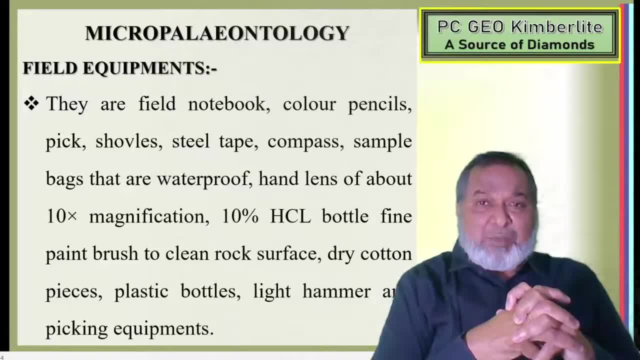 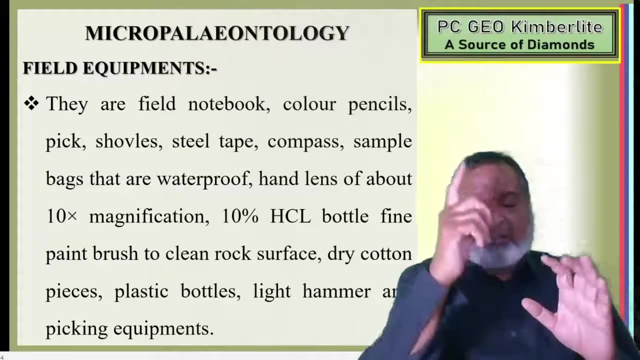 So diary is a very important one. Then the color pencil will be required. Pencils are required, Then the small picks are required, shoals are required. steel tapes are required to measure the uh, the length that you have to measure. the Kleinometer compass, Burton compass are nowadays that we have the GPS is there? 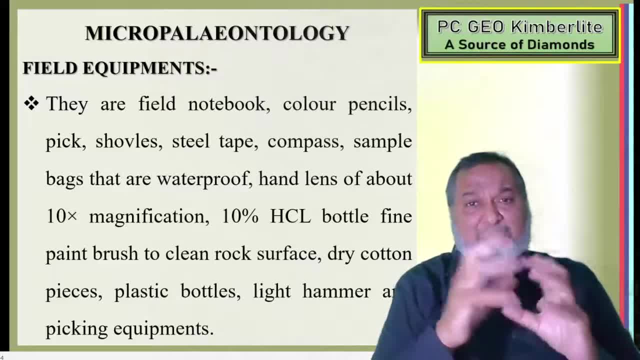 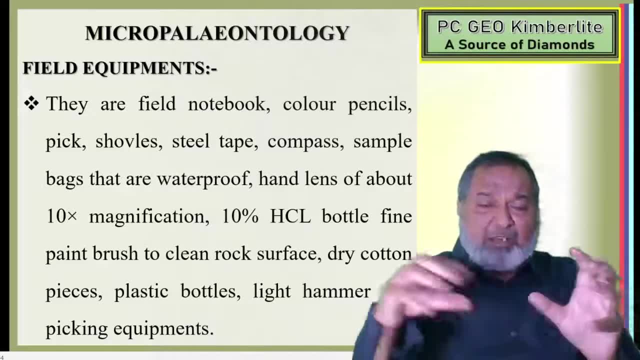 So to make down the proper location of that particular map, these are the compass are required, Then the sample, the Harvard SAC is required. Very important: one Number of uh uh pockets will be there for the cyber side and hand lens. 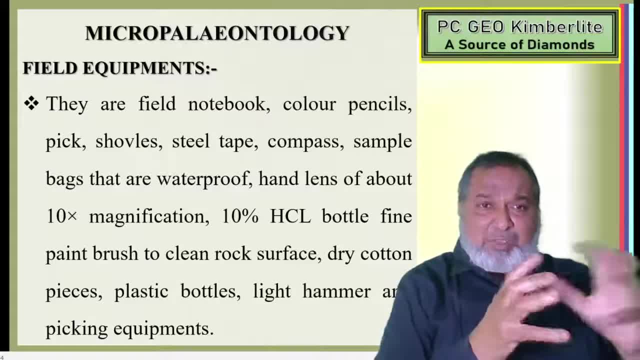 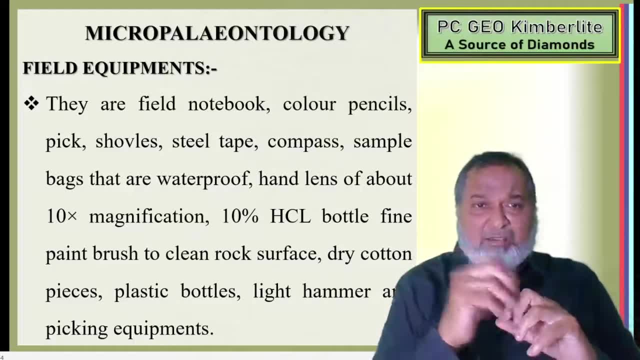 This is the micro fossils are there. So hand lens is there and it has to be 10X magnification, which have how much magnification is there? Then 10% diluted HCL water. fine plastic brush is required to clean the surface brush is required. pointed brush is required. 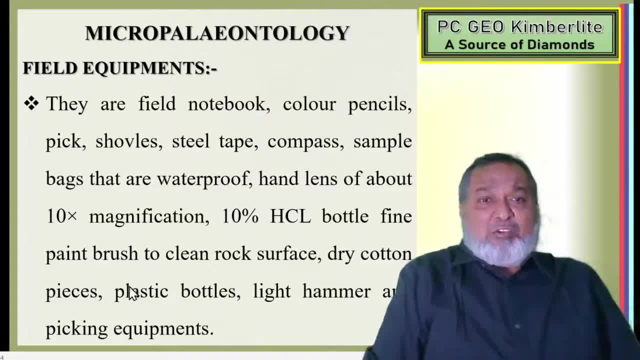 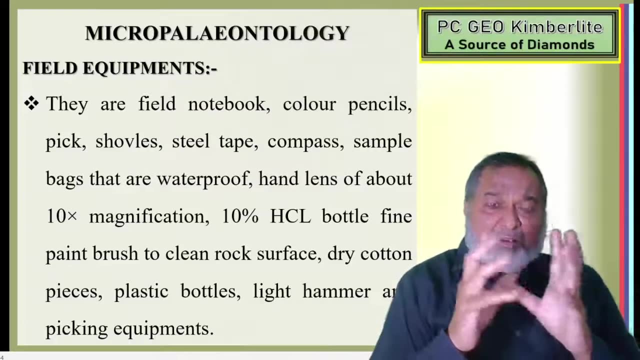 So these are the various type of brush will be required: Dye, cotton pieces, uh, dry cotton pieces will be required, Plastic bottles, Light hammer and picking equipment will be required And, in addition, we require uh uh uh carry bag. 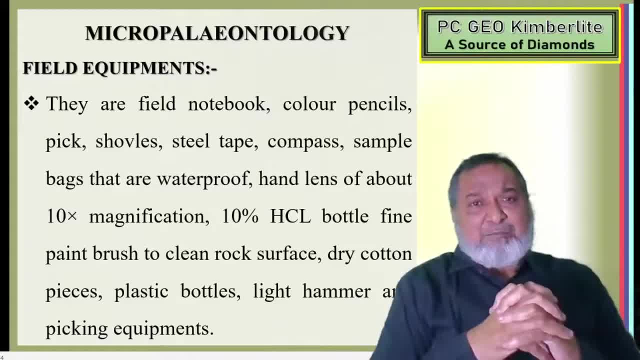 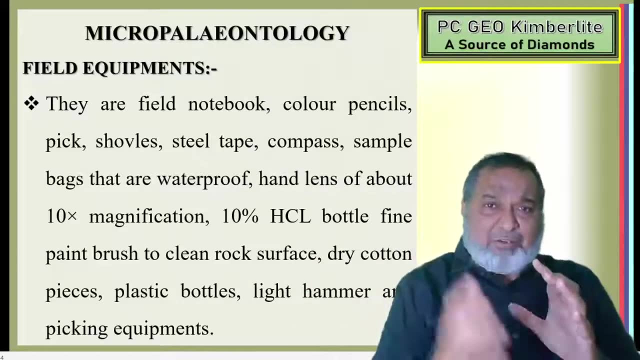 So thick carry bag will be required. How much quantity of sample you want to collect, whether you want one kg or two kg, the friable material is there, rock is there. So on the basis of that we will: frugal material is there. first, clean the surface, weathered material which is there, erode and now fresh rock sample. 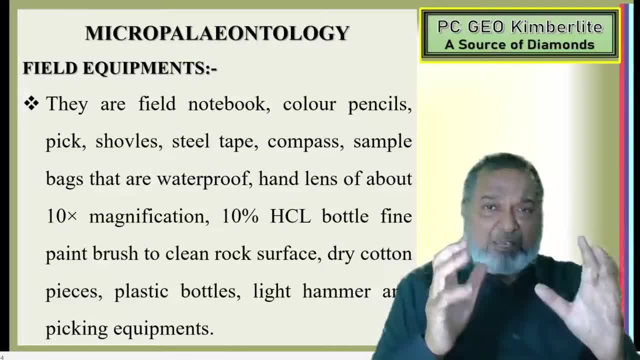 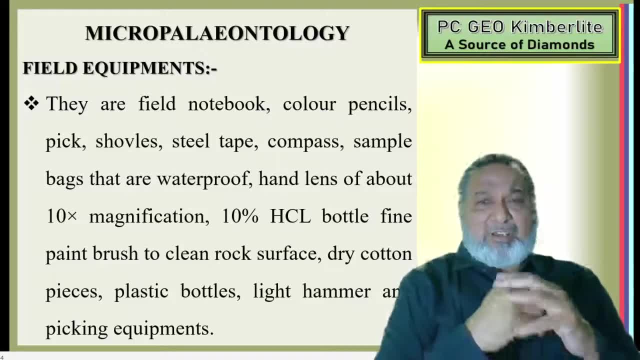 We have to collect so that, whatever the sample which is there, they will be intact and they are not. wear and tear has been taken place, So fresh material has to loose material has to put into the uh, that uh carry bag and uh on the, with the help of the stapler, pin up everything. 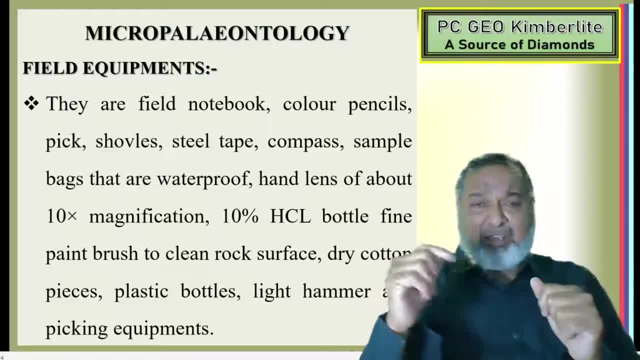 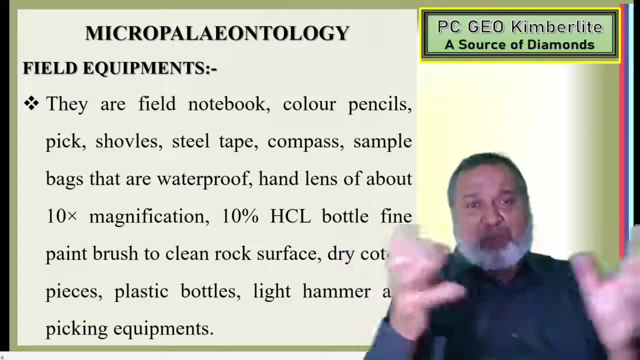 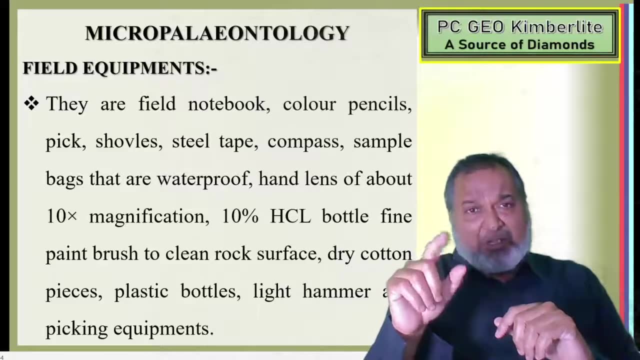 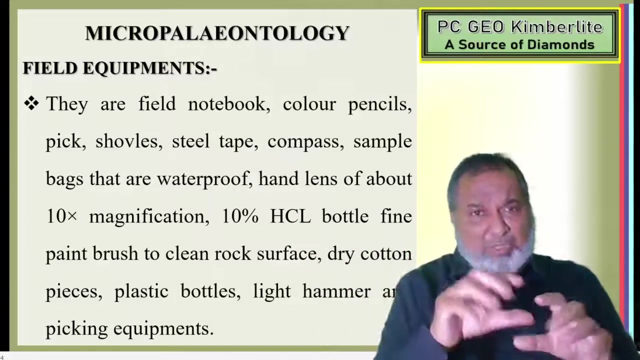 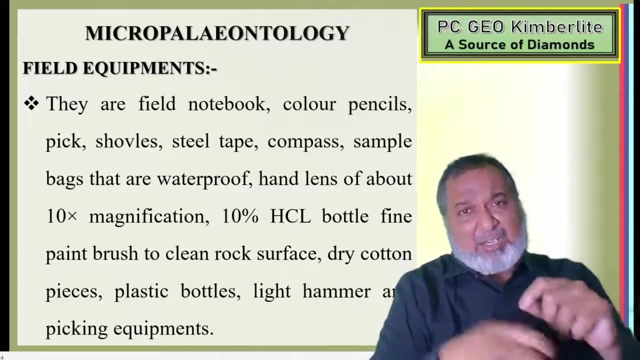 So material should not be come out. write down with a marker pen. the labeling has to done. For example, today is my first uh day, is there? So number of, say, 10 people? So I will write first SH. that is my initial SH, oblique one. that is first location. uh, first day, oblique. first sample, first day, first location. and there itself, whatever I'm going to get down, one, two, three, four of that will be the number that will write down and the same number will be written over there. write down the description in the thing and this thing will be put into the cotton bag. is there tight, that cotton bag? 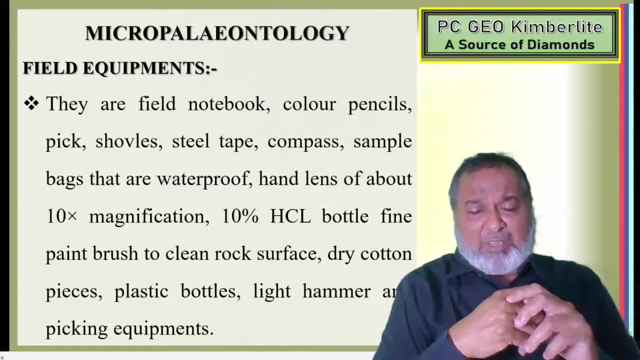 It is uh. so there will be three will be there on that uh cotton bag and on that also with the marker, write down the number and put it into the haversack. It is hard rock. is that directly? can site can put on the number. 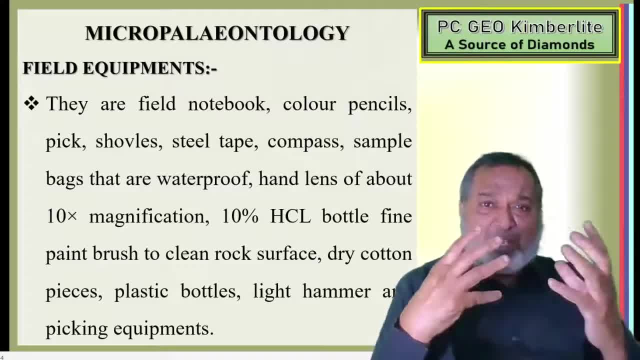 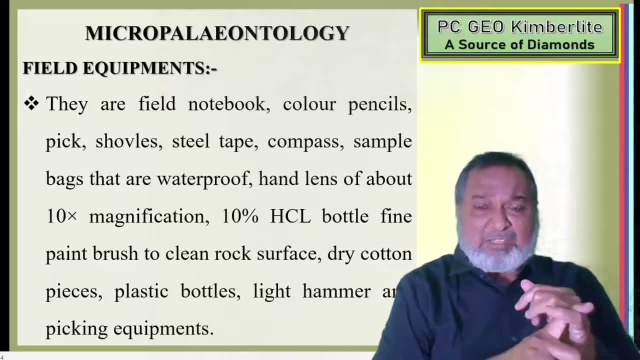 So this will be on the, based on the, what type of rock you are going to get in the field, whether you are going to get a fragile material or it is a hard rock, So that. but then the chisel hammer is required. 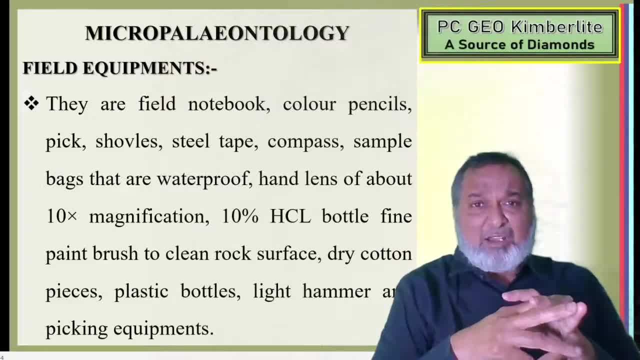 Yes, So these are the things that will be required into the field. In addition to this, if we have particularly a season we have to choose for better for the field work. It should not be a monsoon. It should not be a very hot climate that is in the summer. 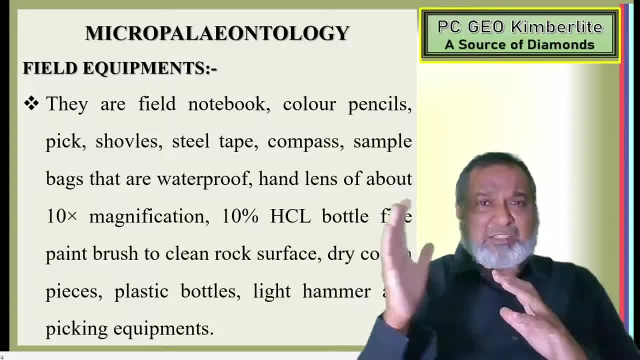 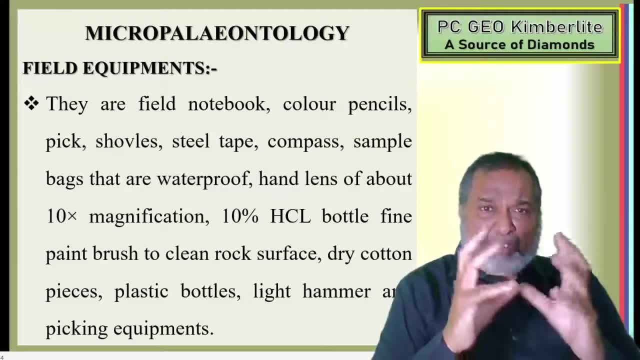 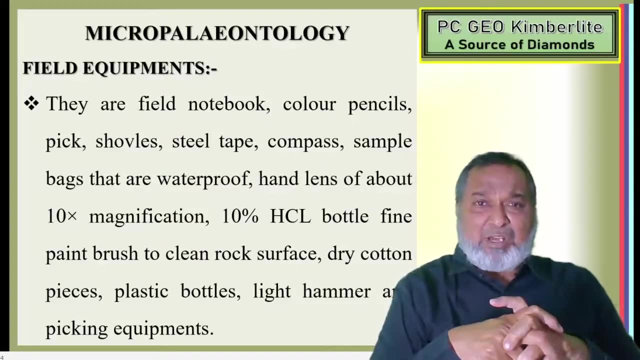 So in between, the winter is going to end and the summer is going to start, So probably in December and the first week of Jan, we will prefer this month for sampling the field, work And early in the morning that will be the best one. 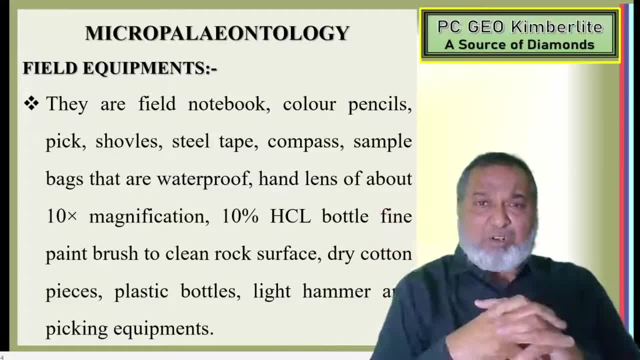 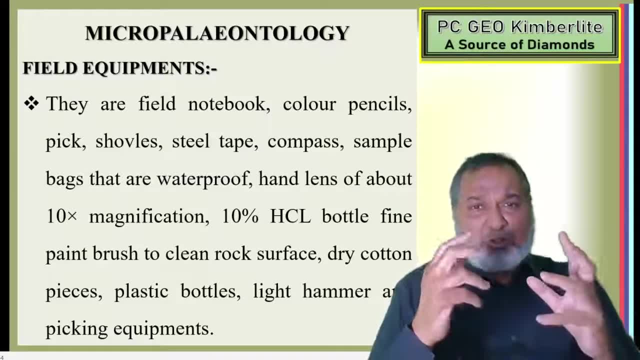 So can finish it out as early as possible- Three o'clock, four o'clock- and complete this work. You're walking into the fields, the terrains are there, So hot terrain, marshy terrain is there, So you have to have the sport. shoes are there. 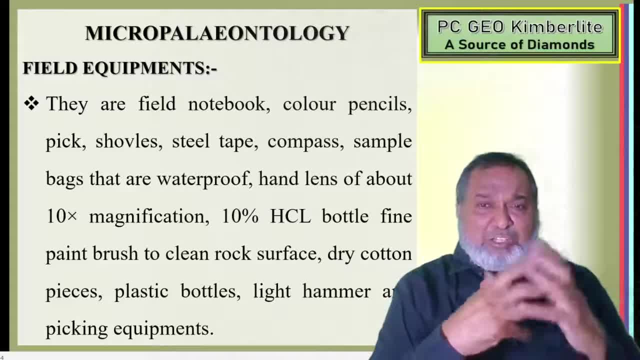 Whatever the pants which you are going to wear, or shirts we are going to wear, They should be a light color. Yes, they should not be a tight one, loose one, sweating should not be there, So they should not be a dark color. 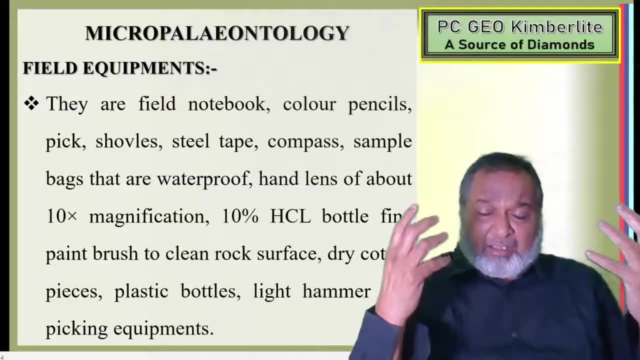 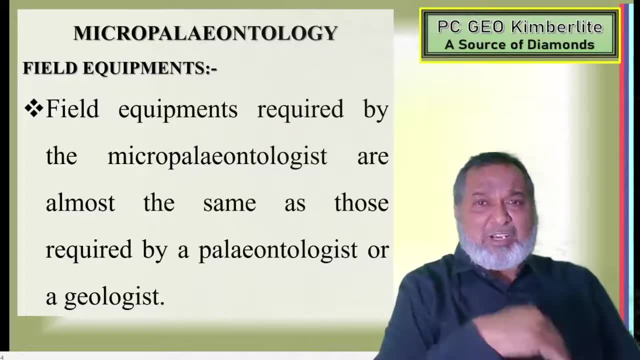 So that also the precaution has to be taken. That hat has to be there. the whatever the pockets are there- there should be a number of pockets- should be there on the shirts as well as on the pants, So that, whatever the climate will come. 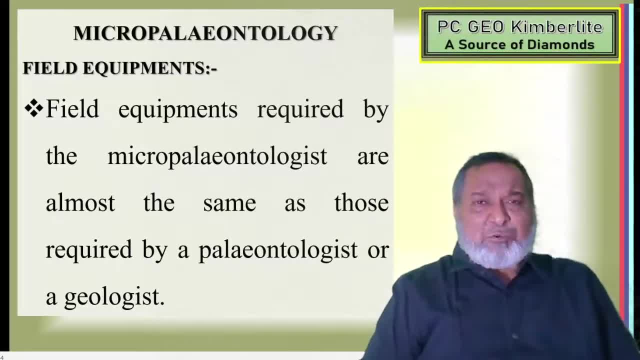 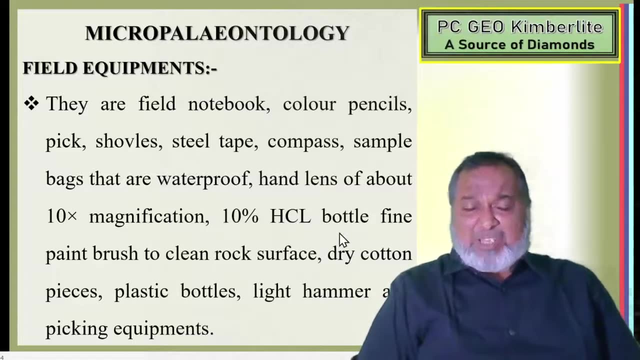 past is, whatever you're going to take it out, put it there itself, So the thing should not be put into the ground So might be able to loose while you're going to the next spot. So that things are very, very important: one when you're going to make out the SEL bottle, which is 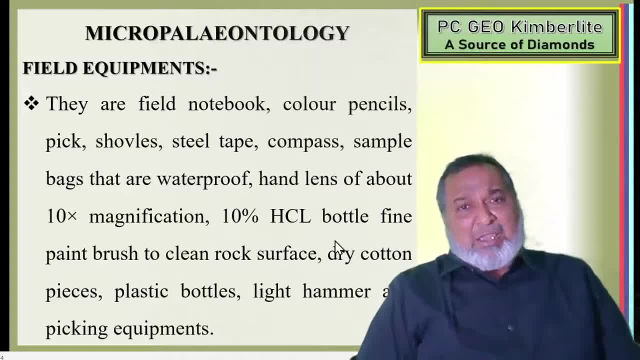 there you have to make a separate one and one drop you have to put onto that rock itself. So if the differences come out, then you can confirm that the rock is the calcareous one, Similarly one if you get the fossil, tiny one put on that. 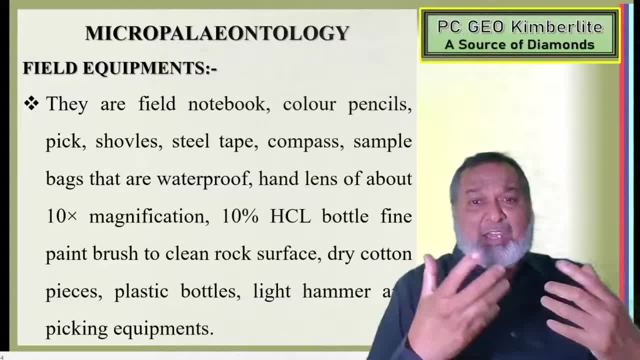 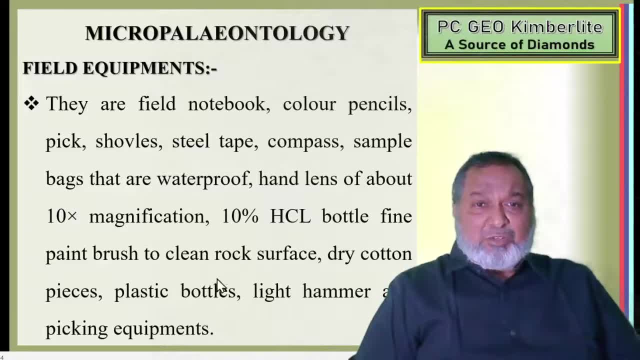 Try to check it out whether it's calcareous or fossil. So you can make up the simple test One norm. that will be the easy one to get the bottle, But that is a very handy one. So water bottle is required. Plastic bottles are also there. 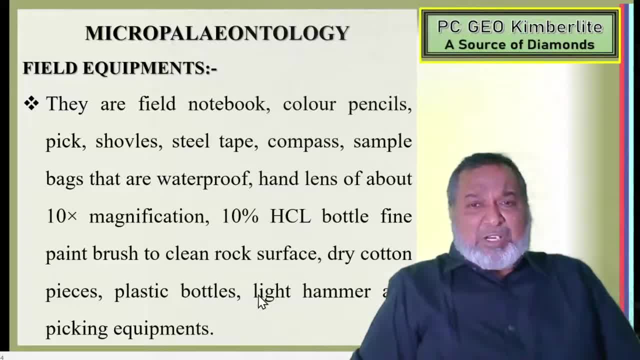 They can feel over there. There's a number on that, So that is their light hammer. Geological hammer is there. That has to be there. In addition, a lot of we require the papers is newspaper, old newspapers- to wrap the material. 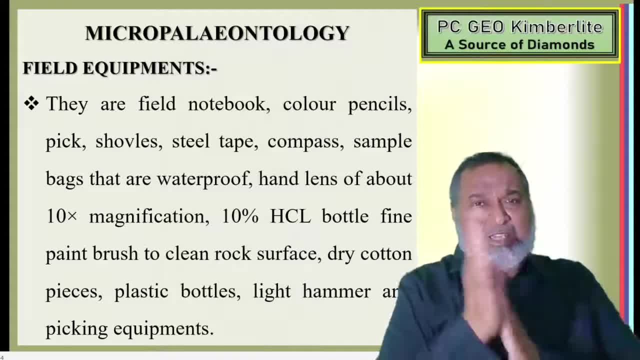 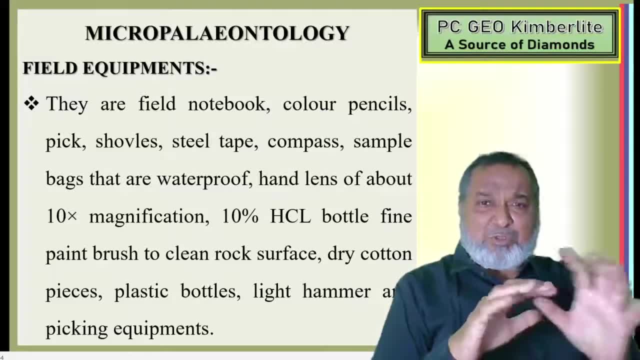 So, while putting to the other side a number of things, you have to be walking, So they should not be there. and there has to be taken place while you're walking, So there should be- you put the paper. So for minimum wear and tear. 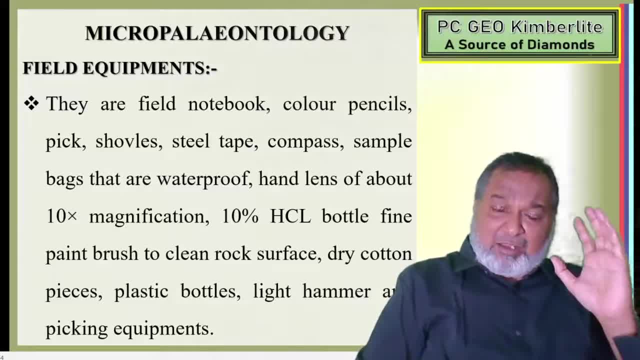 That has to be done. So these things to be there, Then it should be there. Water bottle should be there, Then camera has to be there, A professional camera. If you have the mobile or a high resolution mobile is that, then that will be a good one. 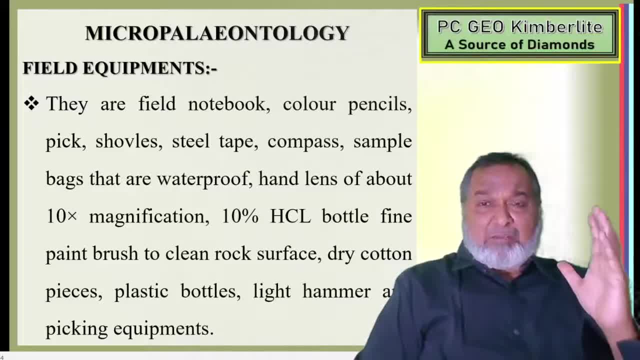 But one thing is that you should not be kept into the field. Take a proper precautions while you're going to the next port. check out Anything should not be left behind, because when you have been going to the next port you're going to show anything is loose. 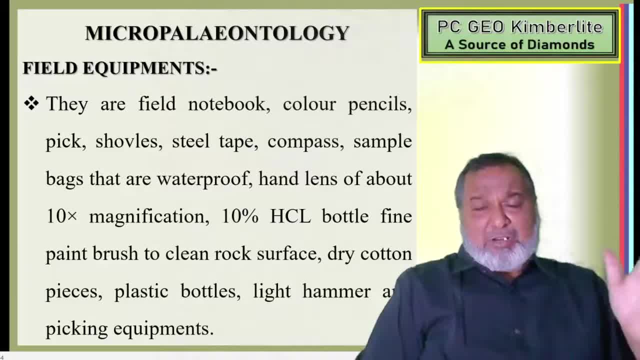 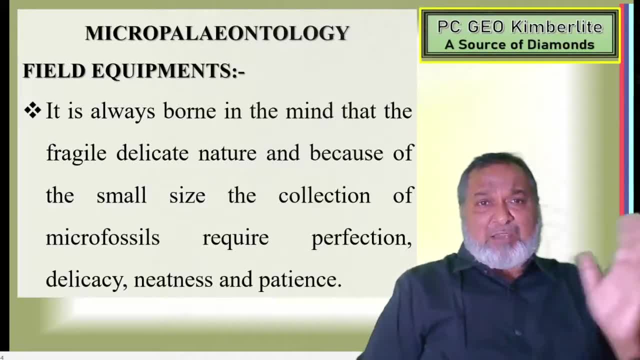 Then we are going to make out your last timing. So planning has to be done properly. So how you're going to make out the things to the field that will be there. So these are the what we have. The things properly has to be maintained. 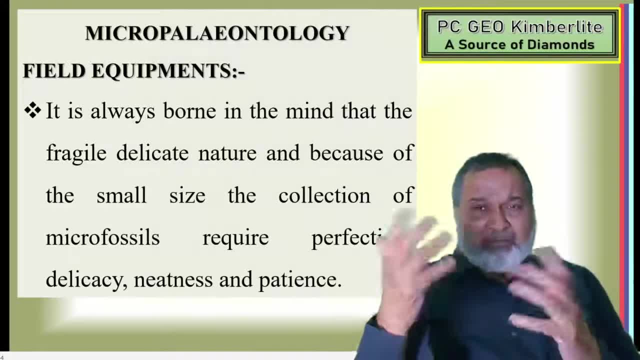 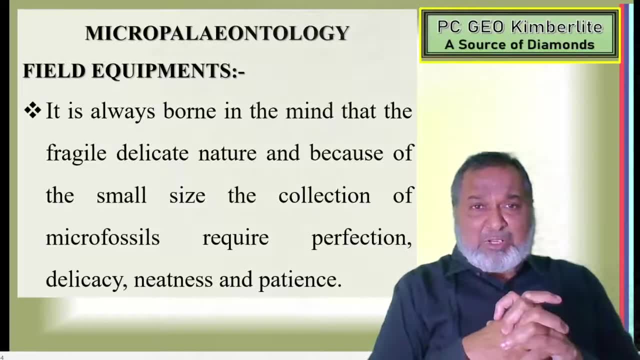 And how many days then sleepers the for the meaning, you have to be there. So the shoes- sport shoes, not a leather shoes- has to be there and not be there. These are the things keep into the mind when you are going for a field work. 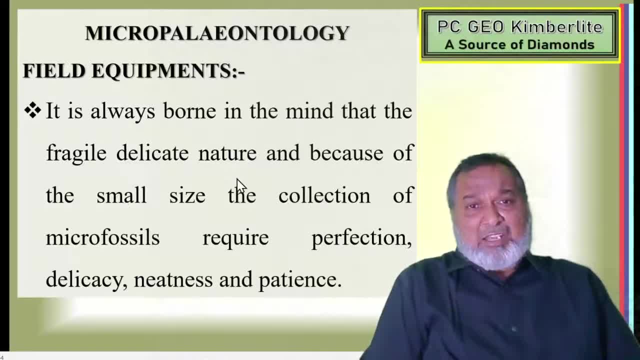 and always born in mind that fragile, delicate nature, And because of the small size of the collection, might require perfection. So yet, perfection is required, Delicacy is required, Neatness is required and, very important, patients are required. So this thing, when you have been sitting over there, properly made a systematic. 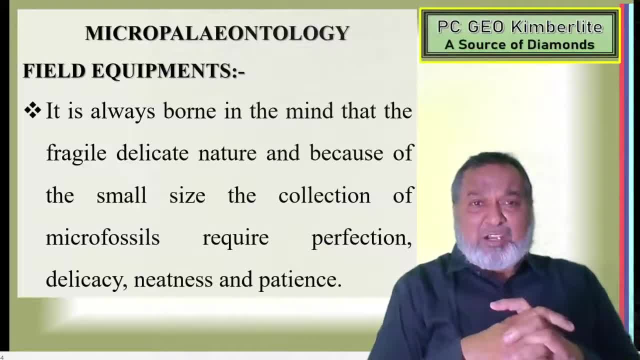 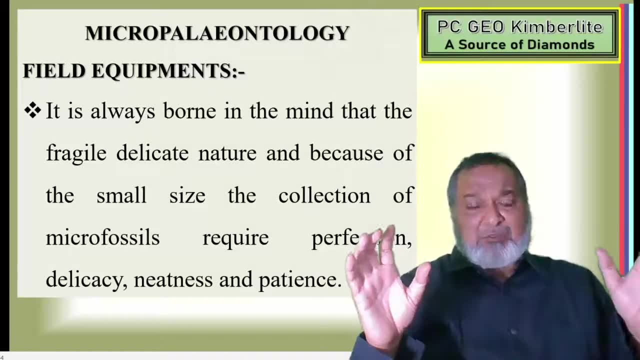 how you're going to feel. there should not be. any contamination has to be done Or whatever the weather material there. from there, The model should not be taken out. It will be a fresh surface. You have to put it out, the hammer in the surface area with a brush and all. 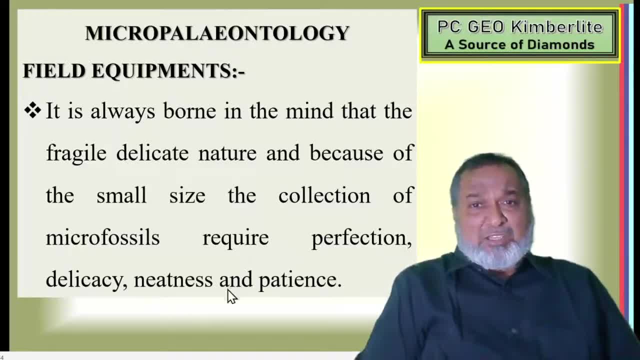 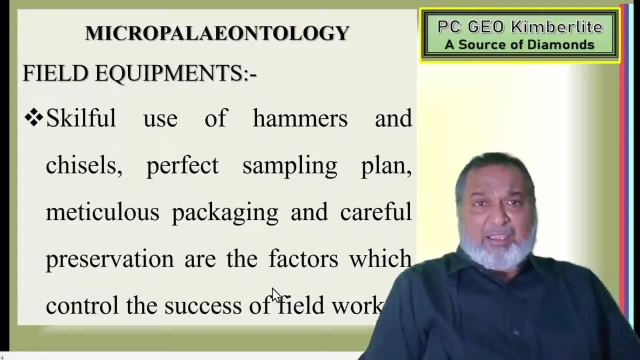 Then from that fresh area you have to collect the sample. So the in the field, you require a perfection, delicacy, neatness and patience, A skillful use of hammer. that is very, very important When you are going to use the hammer. 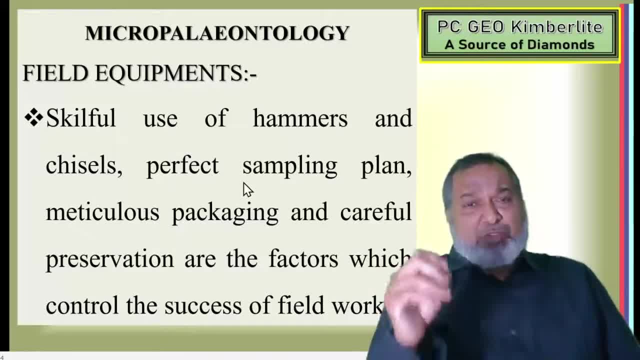 it out. anything Or a chisel, you have to make it out. So you should not be cut the samples When you are going to make it out. use it hammered properly. Perfect sampling plan, meticulous packaging and careful preservation are the factors which control the success of the field work. 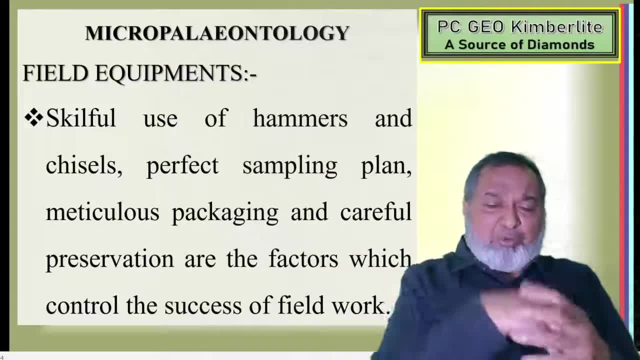 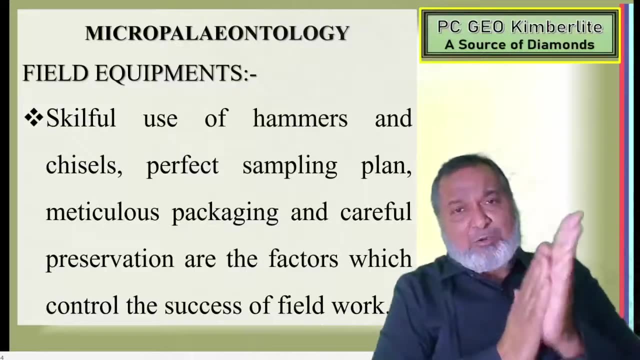 If you're not done properly- and you're not done properly, put it into a cotton bag, wrap it out and after wrapping again with the old newspaper, that will be minimized, or sometimes we'll use the cotton also, so that while in the travelling also there will be wear and tear. 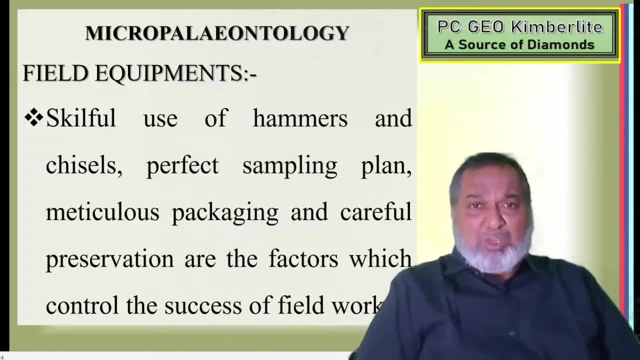 So contamination: two samples should not be mixed. So these are the very, very important ones: Perfect sampling plan, meticulous packaging and careful preservation. These are the three very, very important ones there in the field. So once you've done this one, then your success. 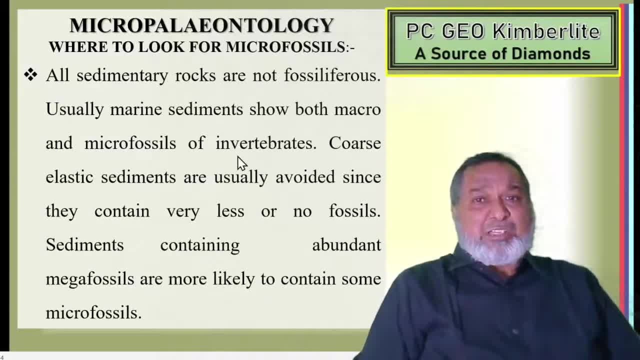 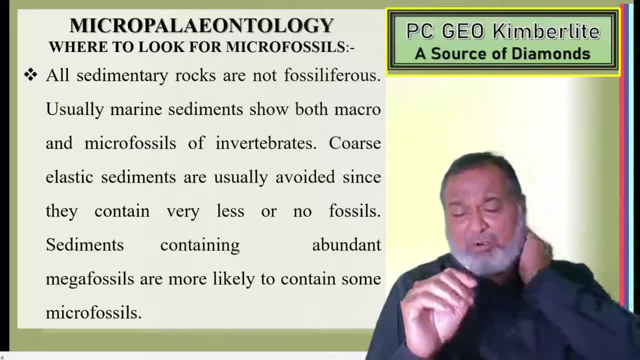 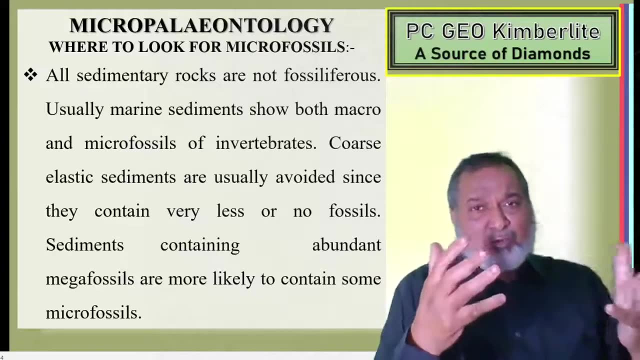 field work will be very nice. All sedimentary rocks are not possible. Keep in mind when you're going for a field work. keep in your mind. every sedimentary rock should not have the fossil. It will be marine sediment. so both micro as well as micro, macro and micro as well. 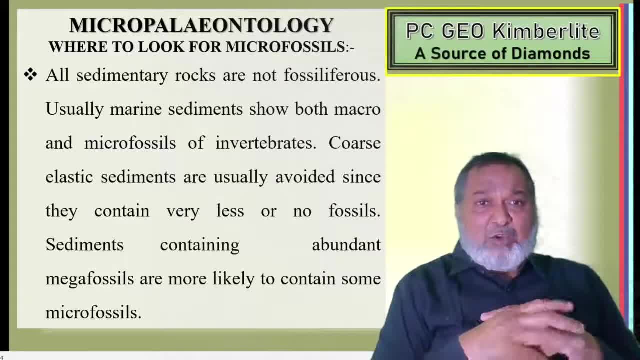 as mega fossil will be there. vertebrates, invertebrates will be there. Coarse elastic sediments are avoided. Yes, whenever you have coarse sediments are there, you have to avoid because there will be less fossilization will be there, since they contain very less or no fossil. 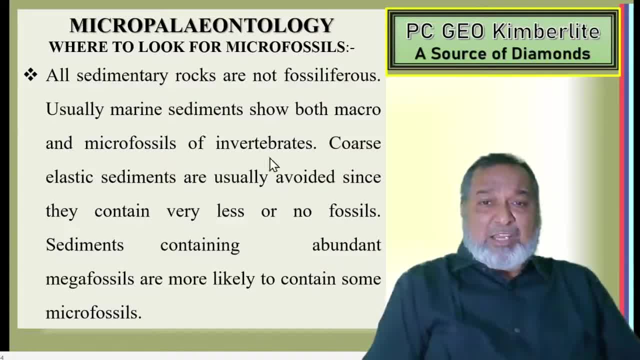 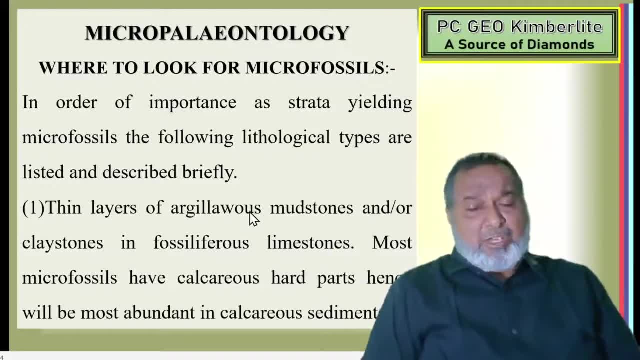 Sediments containing abundant mega fossil are more likely to contain some micro fossils. So that has to be very carefully. you have to observe in the field. You have to open your eyes in the field and observe, plan out properly, think carefully, study properly, make, analyze yourself and try. 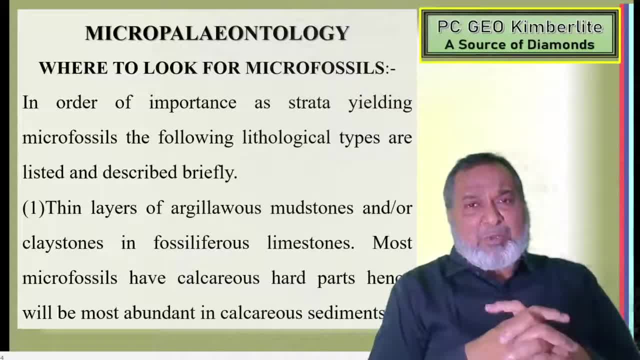 to interact with your subordinates so that the thing should be done properly And whatever you have done, write down in your diaries. That is the very, very important, And where you have to look for the fossils in order to importance of as 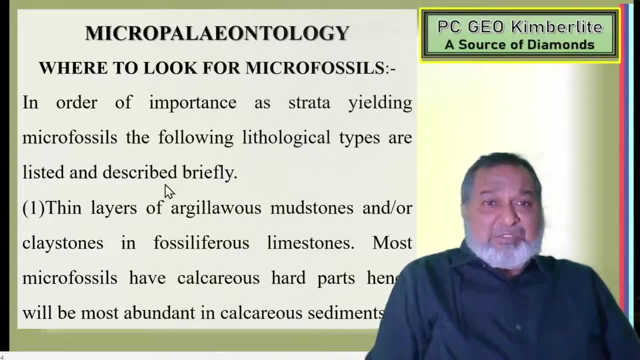 strata-irritating micro fossils. the following lithological types are listed and described briefly. is the first one: thin layers of argillaceous mudstone and claystone in fossiliferous limestone. You have to check for the argillaceous mudstone. 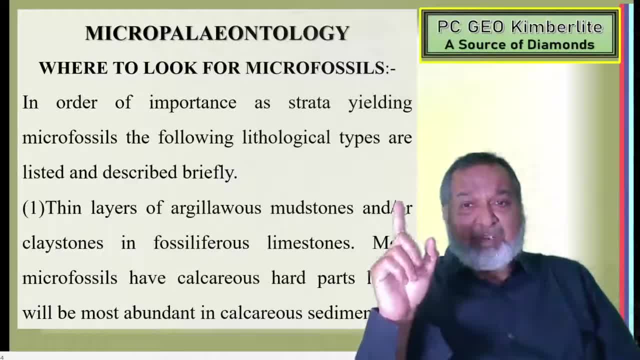 You have to check for the argillaceous mudstone. You have to check for the argillaceous mudstone and claystone. in fossiliferous limestone, Most fossils have calcareous hard part, hence will most abundant in calcareous ceramides. 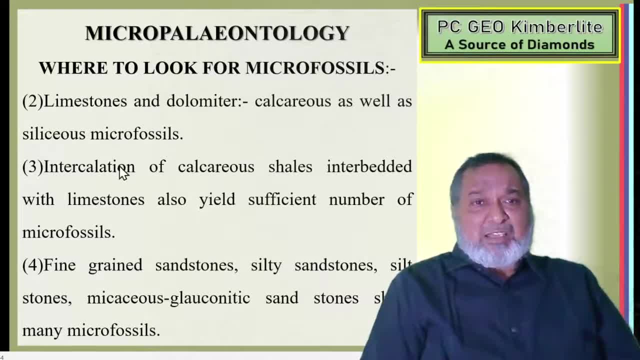 Limestone and dolomites calcareous as well as siliceous micro fossils. In limestone and dolomite, you will get the calcareous as well as siliceous micro fossils. Spelling mistake is there, So I apologize for here. 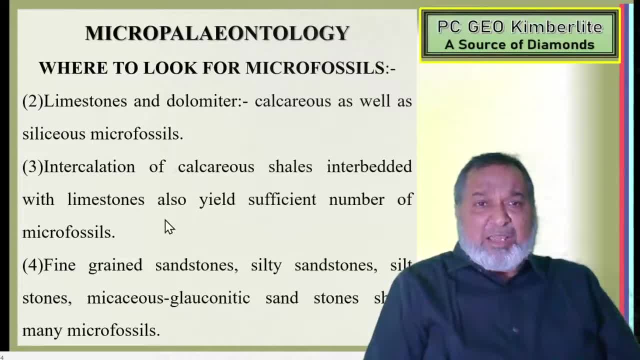 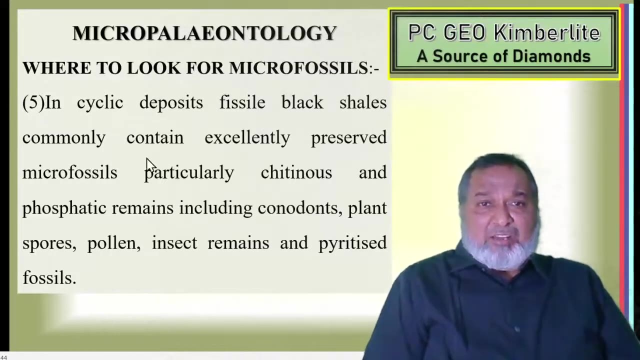 The intercalation of calcareous shell bedded with limestone also yields sufficient number of micro fossils. Fine grained sandstone, silty sandstone, silt stones, micaceous glyco-nagnetic sandstones show many fossils And in cyclic deposit, fissile black shell, commonly contain excellently preserved micro fossils. 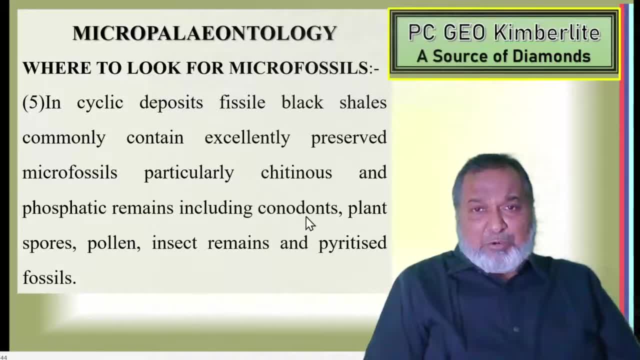 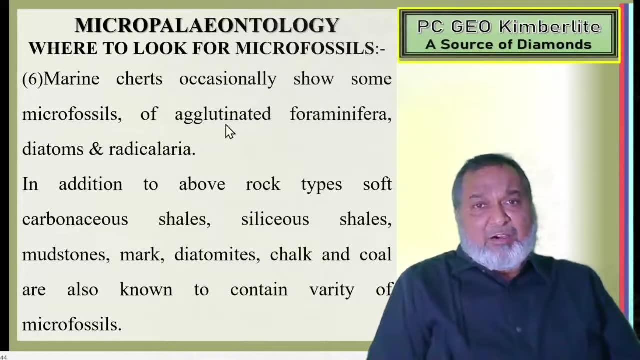 particularly chitinassana. phosphatic remains, including conodotes, plant spores, pollens, insects and remains and paritized fossils. Mudding charts occasionally show some fossils of agglutinated foraminifera diatoms or radiolarias. 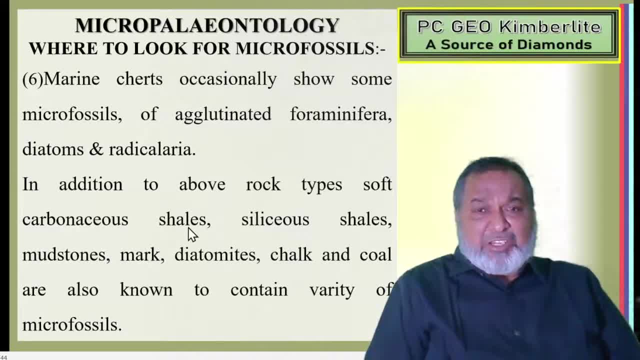 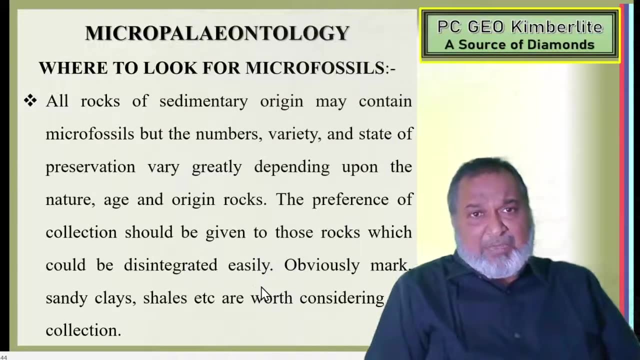 In addition to the above rock types, soft calcareous shells, siliceous shells, mudstone, marl- it is not a mark, it is a marl. dolomite, chalc and coal are also known to contain a variety of micro fossils. 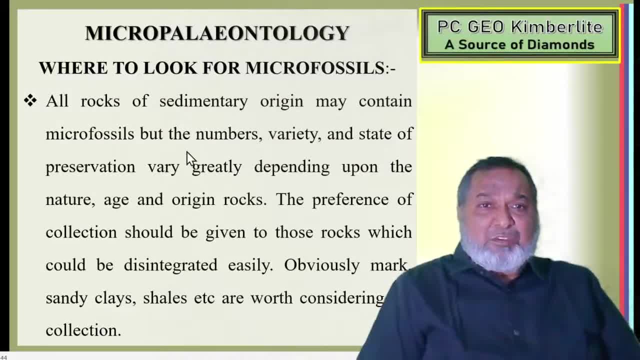 All rocks of sedimentary origin may contain micro fossils. but the numbers and variety, Yes, that is very important. All sedimentary rock which are there in the origin, they contain micro fossils. they are the marine one. Then the numbers, variety and state of preservation is very greatly depending upon. 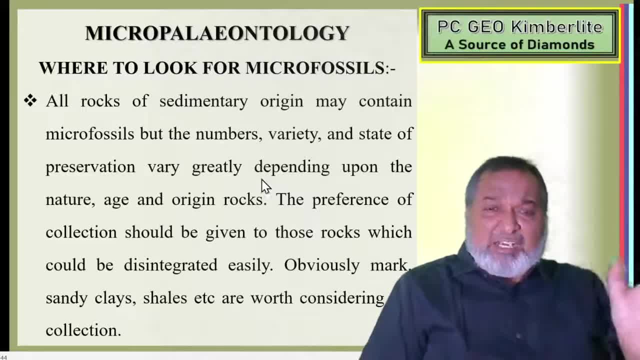 what nature of the, what we have, the test is there. what is the age is there? what is the origin of rock? So these are the things: nature, age and origin. That is a very, very important one for making for micro fossils. 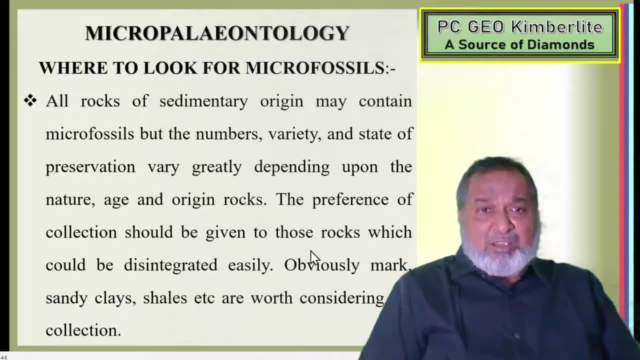 The preference of collection should be given to those rock which could be disintegrated easily. Those rocks which are disintegrated easily, obviously marl, sandy, clays, shells are the worth considering for collection. So, marl, it is not a mark- marl n-a-r-l, sandy, clays, shells, etc. 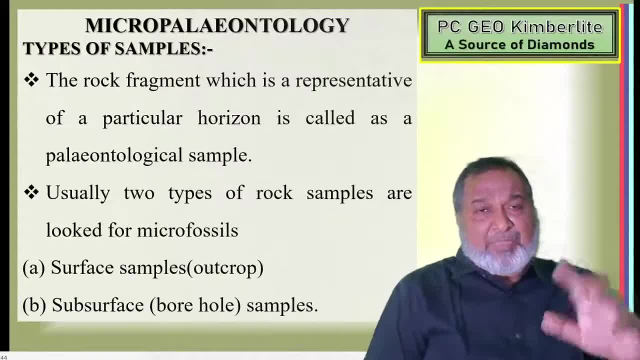 are worth considering for collection. The rock fragments with a representative of a particular horizon is called as paleontological sample. Yes, What is a paleontological sample? Rock fragment is a representative of particular horizon. It is called as paleontological sample. 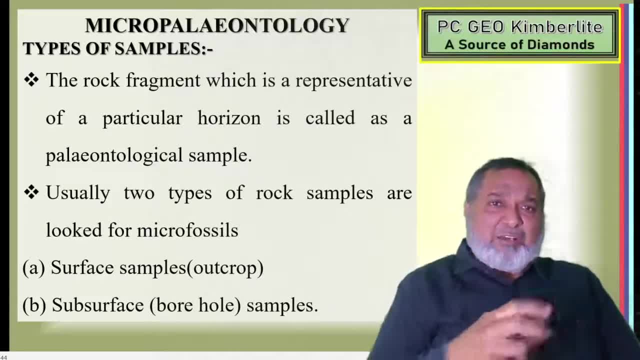 When you are going to collect one sample from one rock, then we have to take the rock fragment of that particular rock and that will be called as paleontological sample. Usually, two types of rock samples are: look for micro fossils. Yes, there are the two types of rock samples. samples are look for micro fossils. 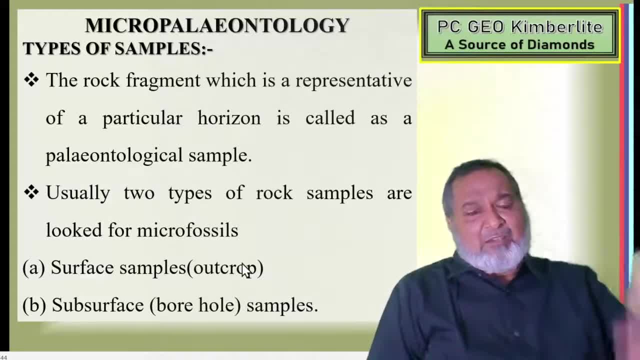 One surface samples That is outcrop. naturally, wherever we go in a road cut or in a river cut which is there and that particular area or landslide which has taken place In that area vicinity, we can get the surface samples or subsurface. 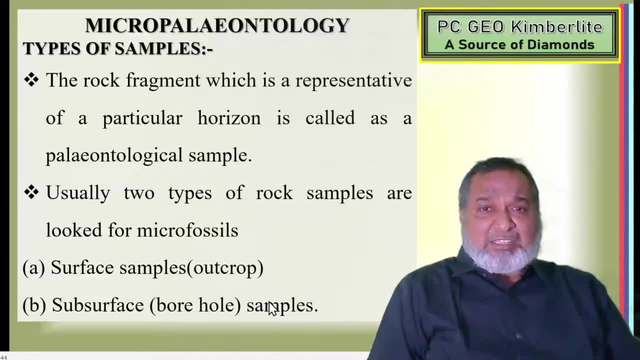 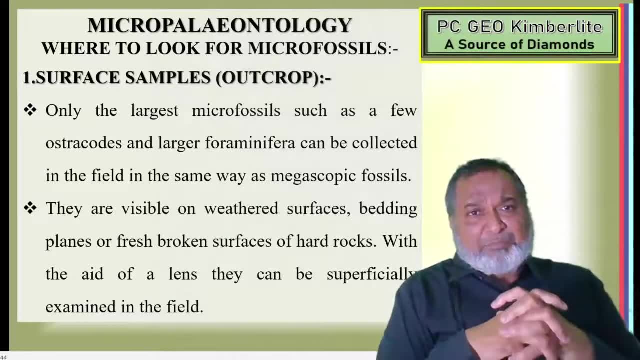 the borehole samples, drilling wherever has done. from that borehole samples we can pick out the micro fossils. First we'll see now the surface sample outcrops. Yes, first we'll see the surface samples. That is, we are going to collect the sample in the outcrops. 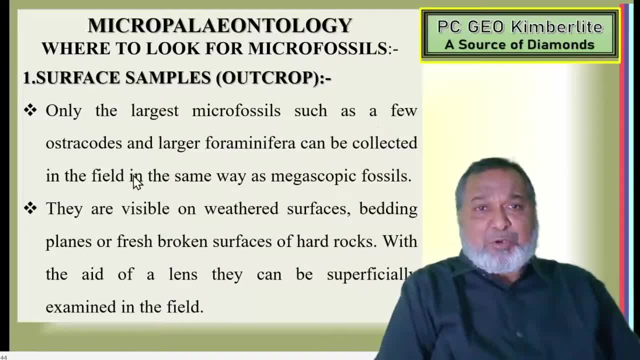 Only the largest micro fossils, such as a few austro-coats and larger foraminifera, can be collected in the field in the same way as a megascopic fossils. They are visible on the weather surfaces, bedding planes or fresh, broken surfaces of hard rocks With the aid of lens. 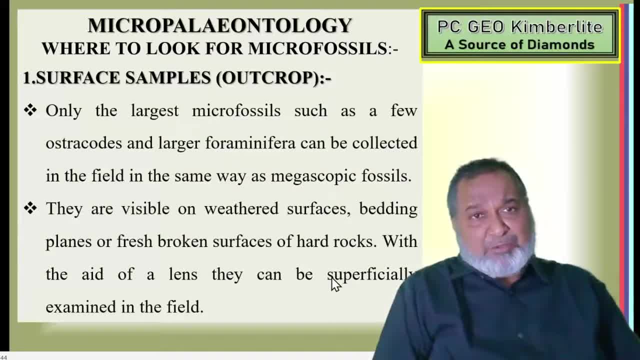 they can be Superficially examined in the field. So this is the way: once you go into the field, you're going to see the weather. rock areas are there, In that you have to go and check it out. bedding planes. 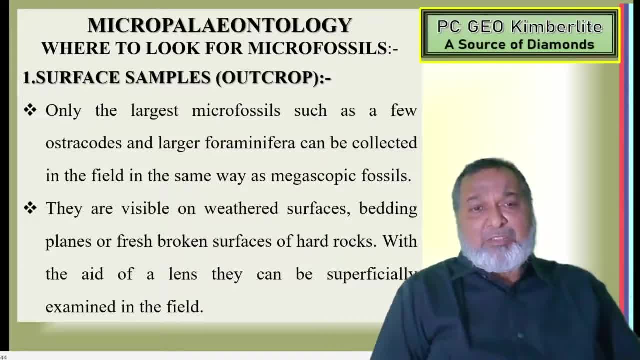 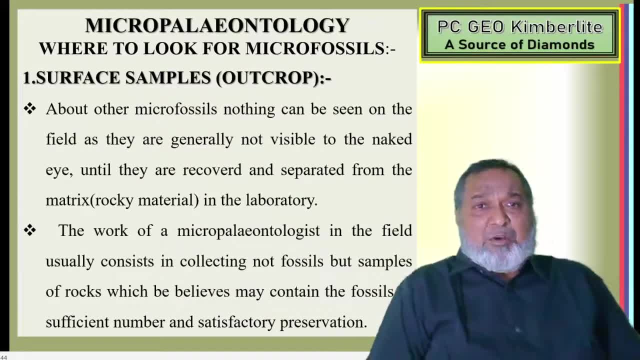 fresh, broken surface of the hard rock and there, with the help of the hand lens, check out, examine the micro fossils. About other micro fossils, nothing can be seen on the field as they are generally not visible to the naked eye until they are recovered and separated from the matrix. 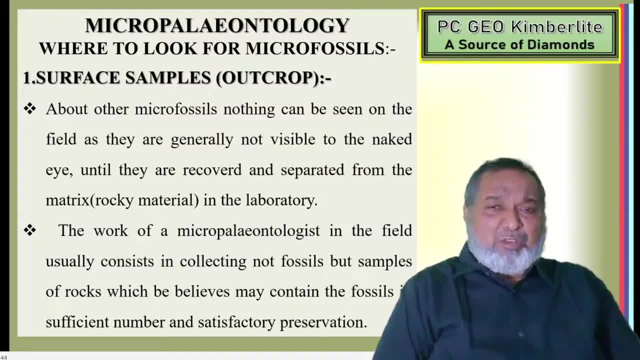 That is a rocky material in the laboratory. So those material which we could not see, the micro fossils with your own eyes, We could not do anything, unless and until we collect them, we separate into the lab from the matrix and then under the microscope we can observe. 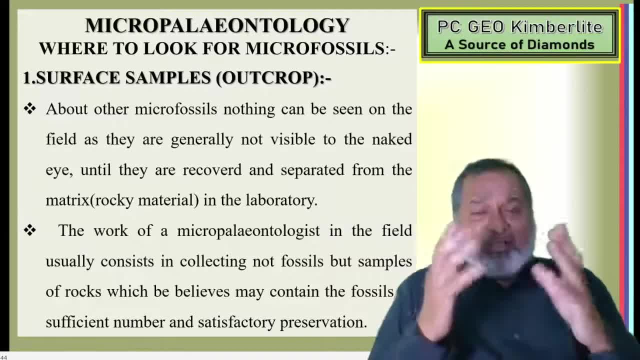 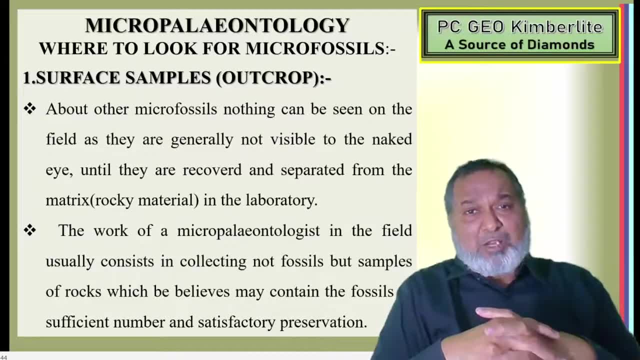 Then we'll come to know whether, whatever the sample we have collected in that sample, any fossils, micro fossils we have got. So that is, once you got it is we are going to get a good, lucky one. The work of a microbiologist in the field usually consists in collecting, not fossils. 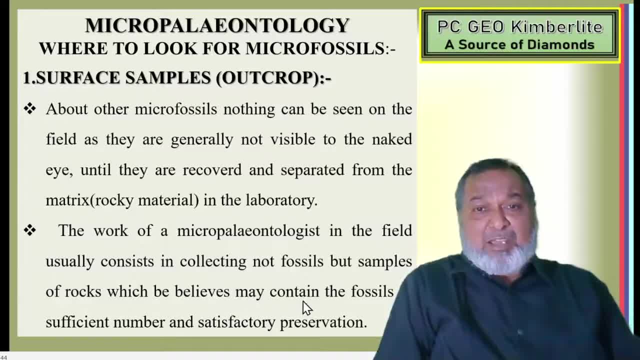 but samples of rock which we believe may contain the fossils. That is the belief that the sedimentary rock contains the fossil. So that is the belief is there. So that's why we go into the outcrop and we are going to search for the fossil. 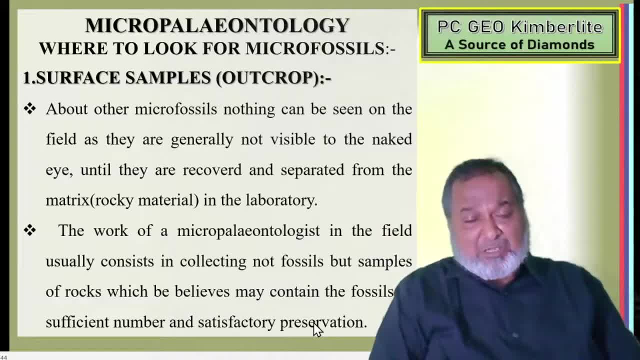 in sufficient number and satisfactory preservation. That is the two things, That is, we should get a sufficient number as well as the satisfactory preservation. Whatever the pre-existing micro fossil is there that has been preserved in that particular rock. So we have to believe this is the microbiologist's belief, is there? 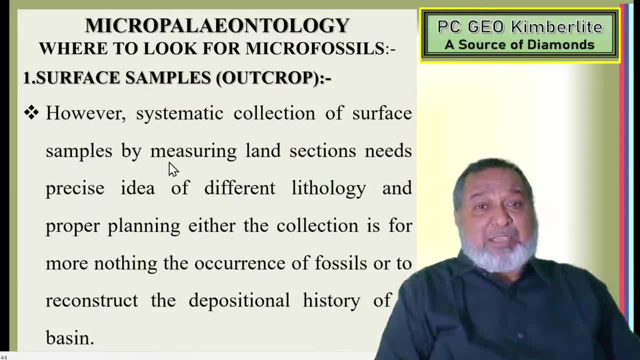 However, the systematic collection of surface samples by measuring land section need precise idea of different lithology. First we go into the section just see that. you will come to know from the colors what type of lithology is there in the vertical as well as horizontal succession. 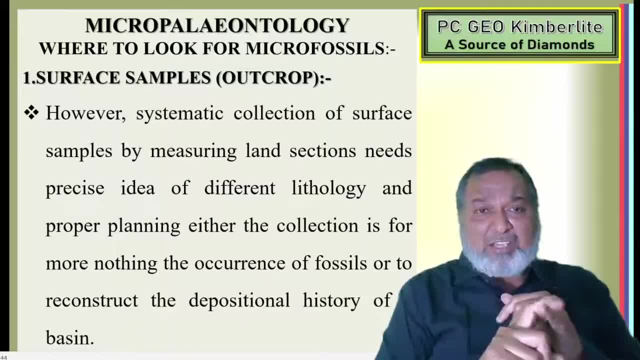 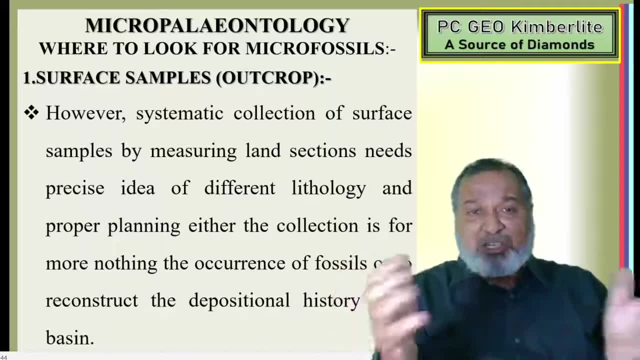 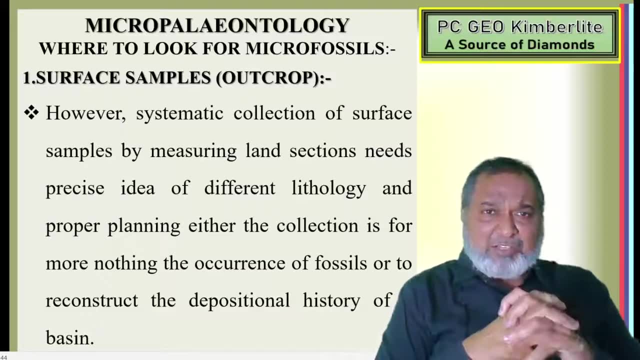 So you have to make the proper planning. Either the collection is for more nothing of occurrence of fossil or to reconstruct the depositional history of a vessel. So keep, when you are going to make out these things, that what is your plan. is there, Just go on. 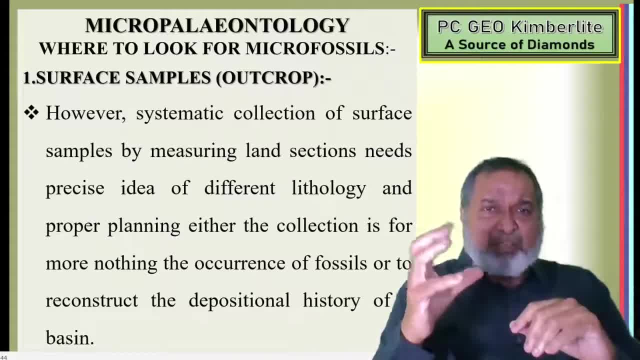 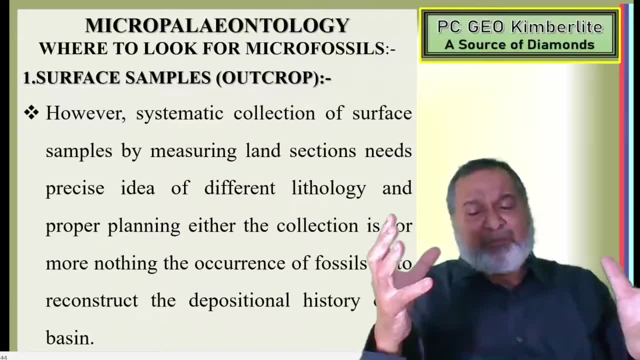 On collecting the micro fossils, or once you are collecting the micro fossils from each bed, then what will be your aim? is there? Not only just we have to collect the samples, separate from the micro fossil, from the matrix, and once you collect it, we just want to know what are the fossils? 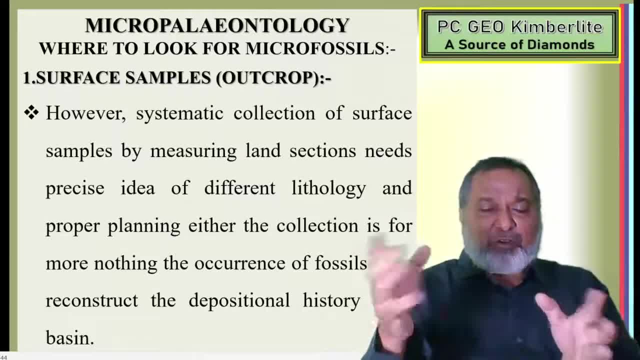 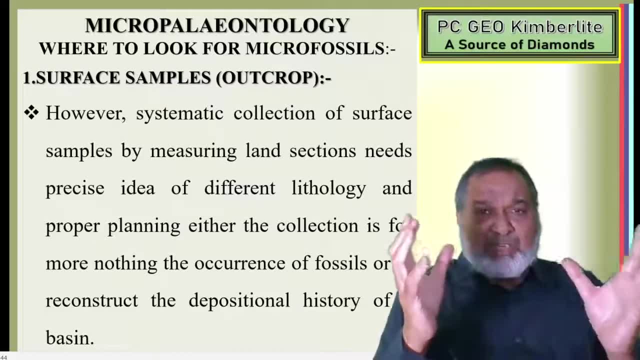 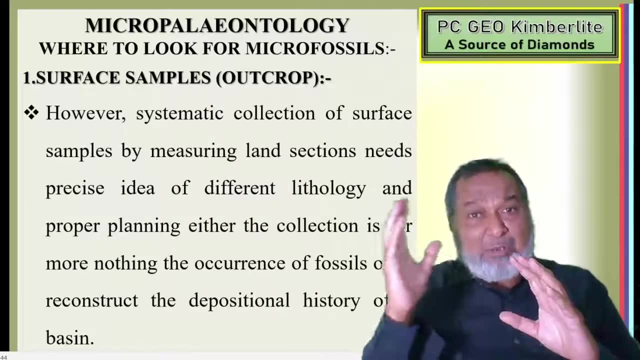 we got, and what will be? the morphology is there, then taxonom is there, So that will be not a big issue, But the important one. if you have, these sediments are deposited And the fossils are formed. So what will be the value of environmental conditions, climatic conditions, 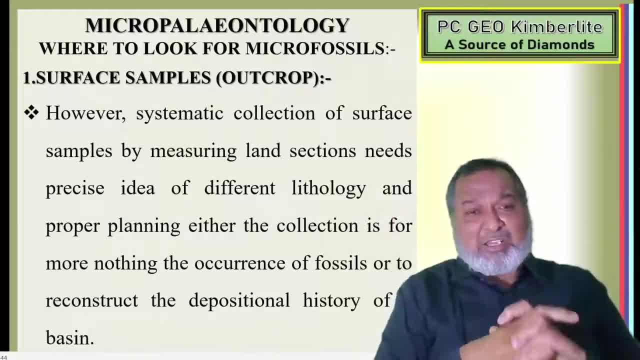 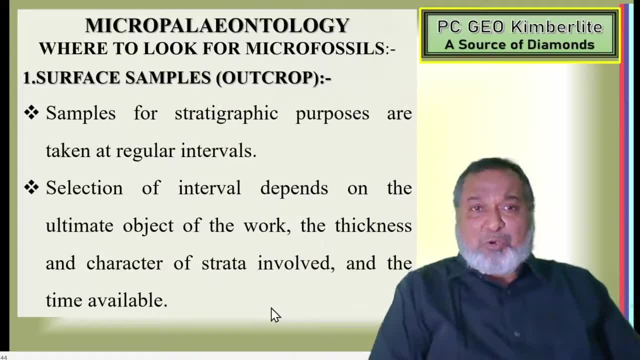 So we want to study that, So depositional history, how the fossils are or construct, the depository history of a basin. So that is a very, very important task for the micro fossils. The samples for study, graphic purposes are taken at a regular interval. 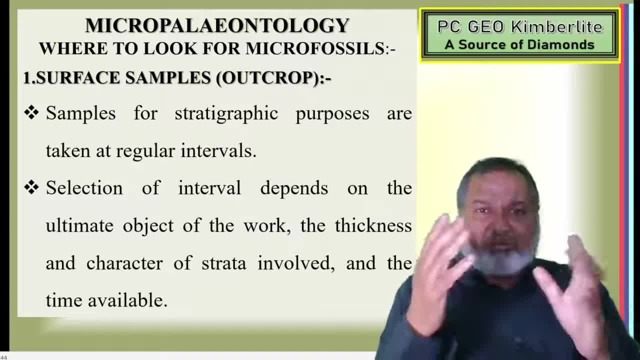 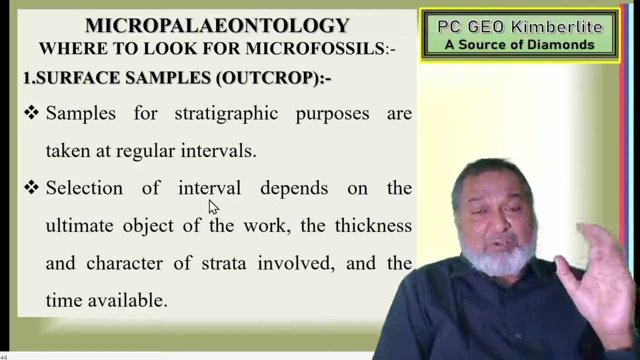 If you are planning is there in a study graphic purposes. is that so study graphic technique you have to use? So which sampling technique we have to use into the field based on our aim? That is a very, very important one. Selection of interval: selection of interval depends upon the ultimate object. 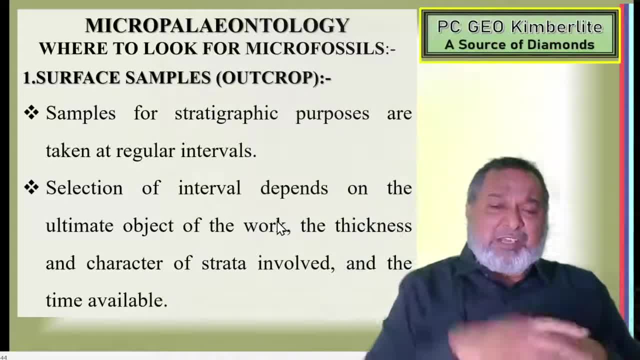 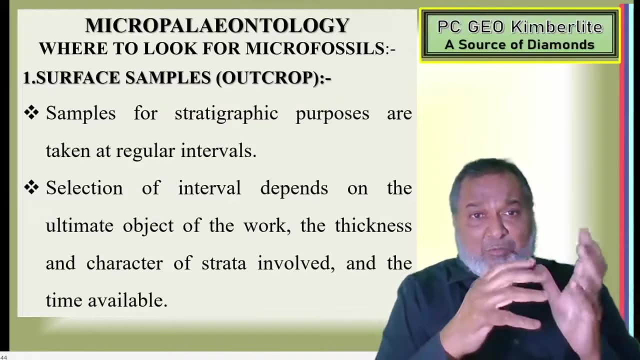 of the work is, say, example, within a 10 feet There are, say, 30-40 beds are there which are. thickness is very less, But now, once you are starting collecting a sample from a thin layer, then how many are there, then what will be there? 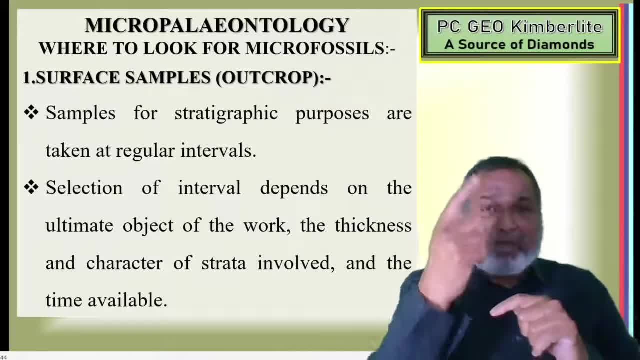 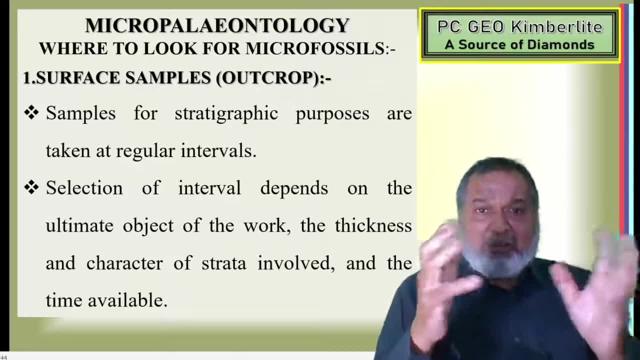 So, ultimately, what is our aim is that, how much should be the interval and what regular interval have to collect the sample? that is a very, very important one. Selection of the interval, that is there. Then the second one: thickness. what will be the thickness of the beds? are there? 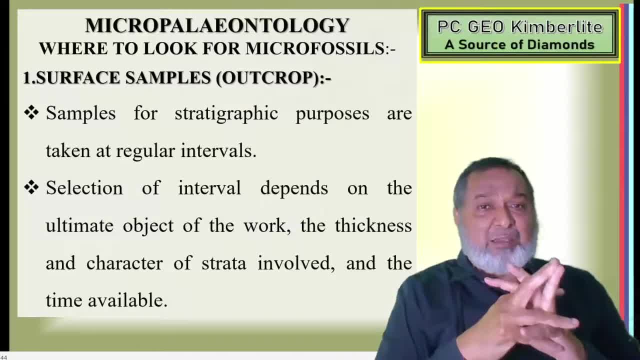 Character of the strata involved and the time available. So how much time is available With the for the collection of samples and what will be the intention is there behind the collection of sample? it has to be clear and broad so that it can get. 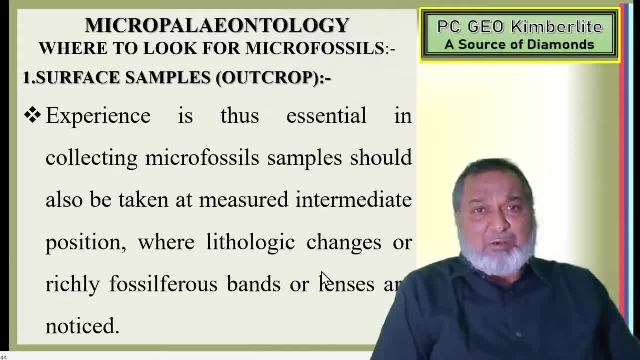 the technique properly and we have to start working on that Experience. that is a very important one. Those experienced paleontologists are there. They have already gone into the field. They have collected a number of times the microfossils and along with them, the new. 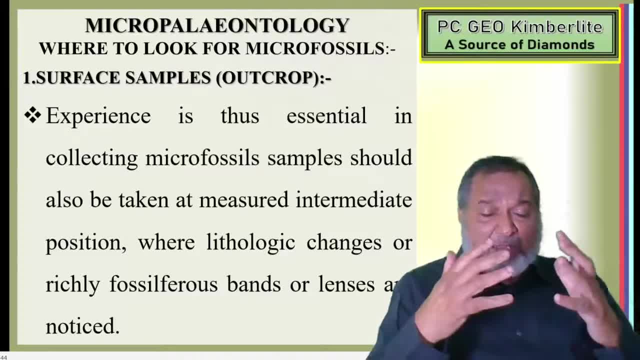 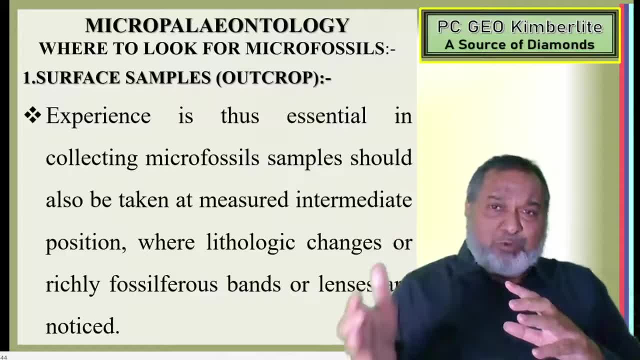 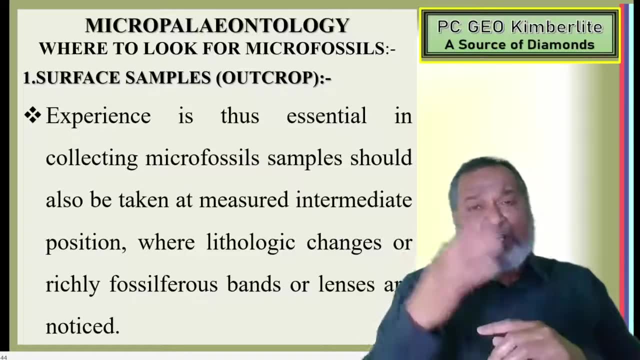 research tools has gone, so they can understand how this geologists are doing a fieldwork in the planning and the experts, the teachers, has to tell them that this is the exposure. is that then? what are the techniques? are there, how many techniques are there and which technique we can apply in this particular section? 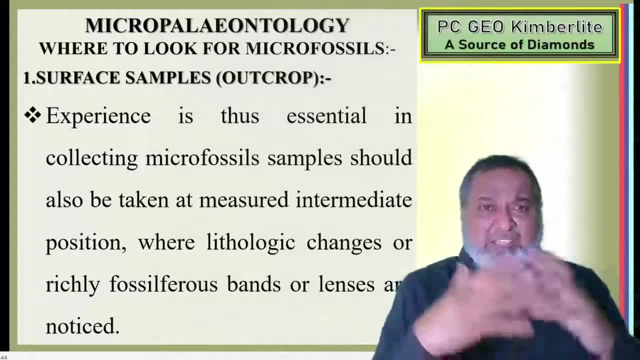 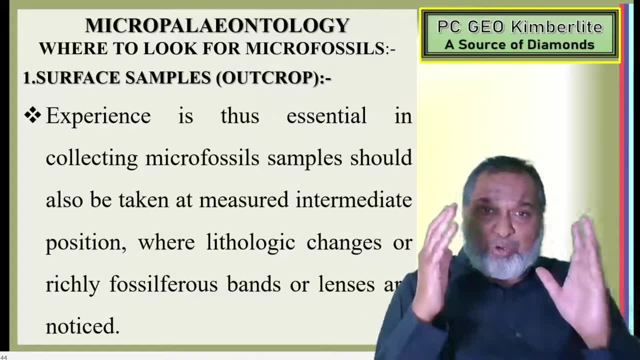 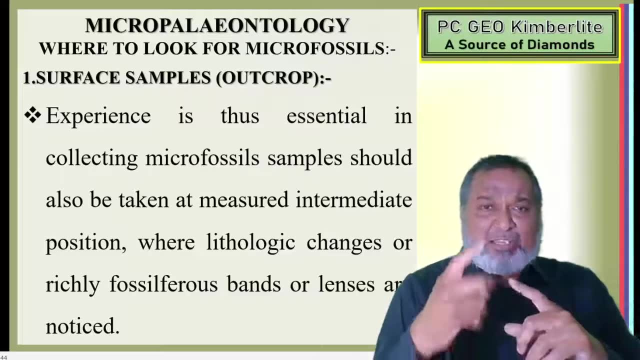 Because that maybe you're going to get in a one day- four, five, six section You may visit and each section may have the different techniques you have to apply. So that technique you have to teach them And at the same time tell them how to collect the sample for sample. 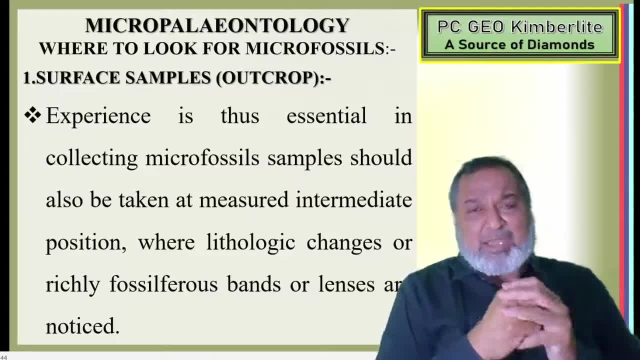 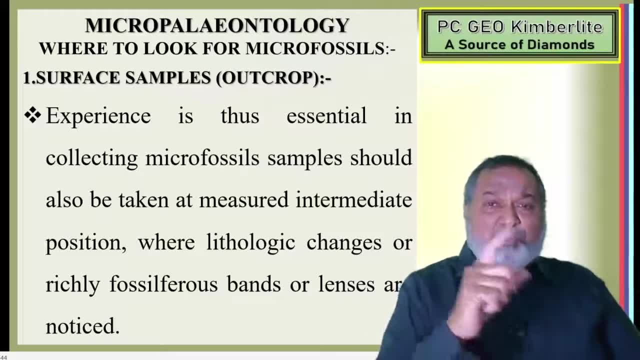 He has to collect and how he has to collect and put it into the bags and properly labeled and keeping, properly into the house that he has to teach to the school, So that students also done the same with the same precautions They have to take meticulously. 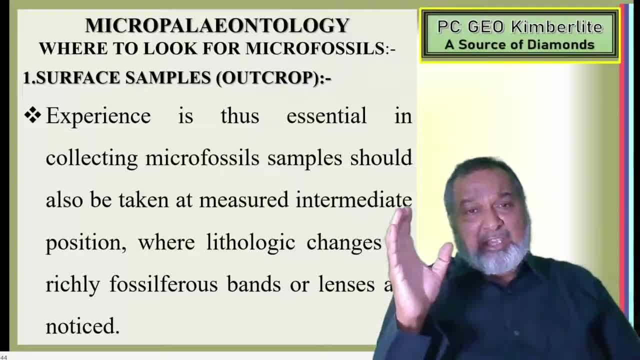 They have to do it and get the patients very important one. You have to teach them the patients that take the time But do it properly, systematically and arrange properly and make carry them in a proper fashion. So the experience is the essential in collecting the micro. 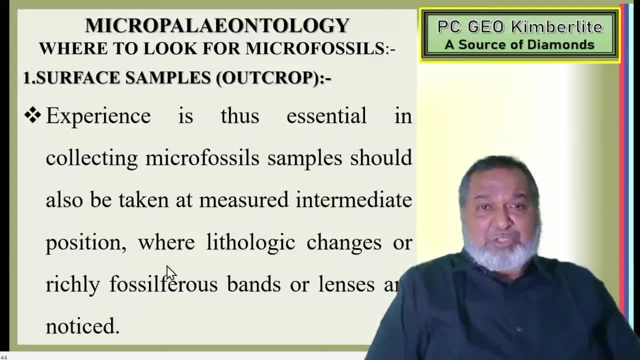 sample should be taken at a major intermediate position where lithologic changes and richly fossilized bands or lenses are noticed Anywhere in the field. Once you're going to see or observe, you'll find out. so many changes are there in the field. 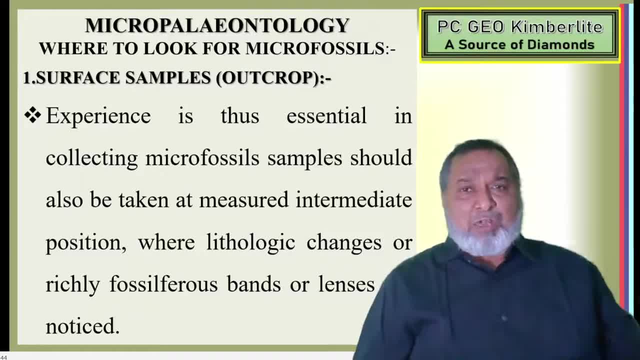 Within this bed that maybe the fossiliferous- sometimes we don't- We don't have the fossiliferous bed- is also there. So what technique you have to use, what planning has to be done, how you're going to make out the lithological changes, the richly fossiliferous bands. 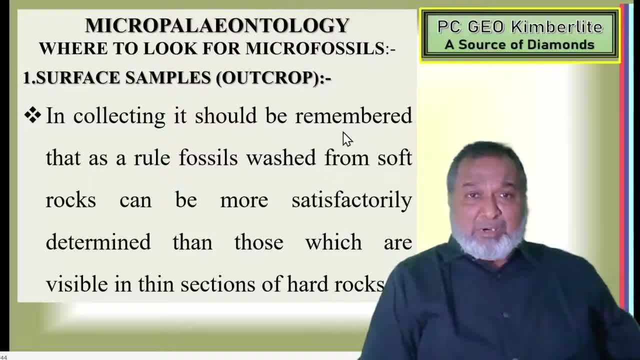 So you have to find out in collecting- It should be remembered- is when you're going to collect them. Remember that, as a rule of fossils washed from soft rocks can be more satisfactorily determined than this Those which are visible in thin sections of hard rocks. 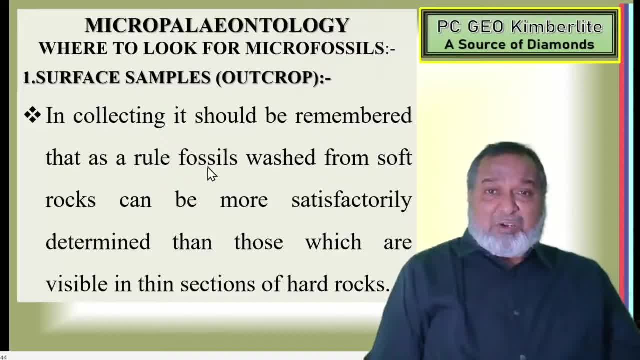 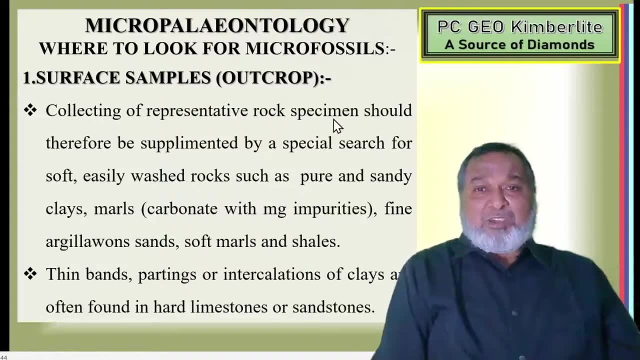 So that is the very remember that rule, that fossil washed from soft rock can be more satisfactorily determined than those which are visible in thin section in the hard rocks. Collecting of representative rocks specimen should be therefore be supplemented by a special search for the soft. 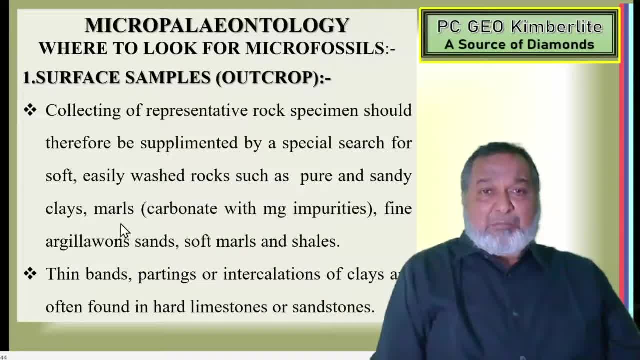 rock. These are easily washed rocks such as pure and sandy clays, marl carbonate with NG impurities, fine argillaceous sands, soft marls and shells. Thin banks, partings or intercalations of clays are often found in hard limestone and sandstone. 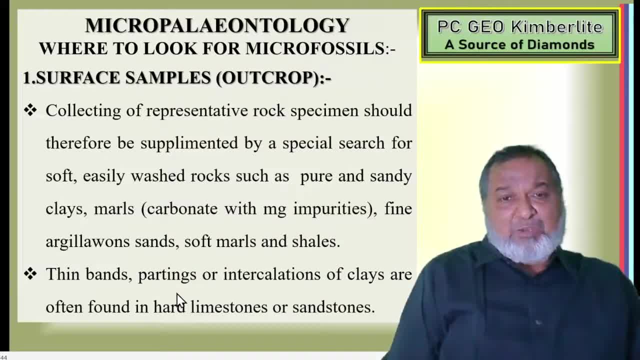 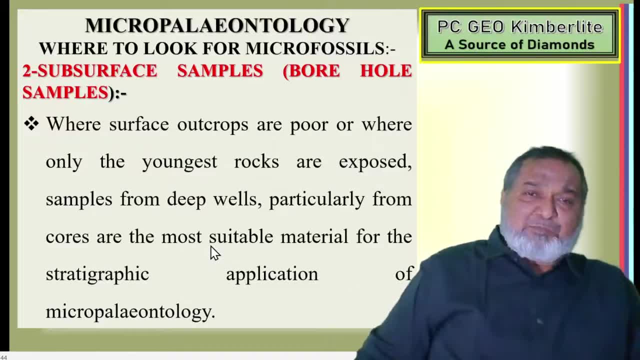 So intercalation of clays will be found in the limestone as well as in the sandstone. So this is the observation And every time the experts teacher has to be give them the feedback that these are the observation. they have to observe and everything has to be note down in the diaries and sketches, photographs they have to take properly. 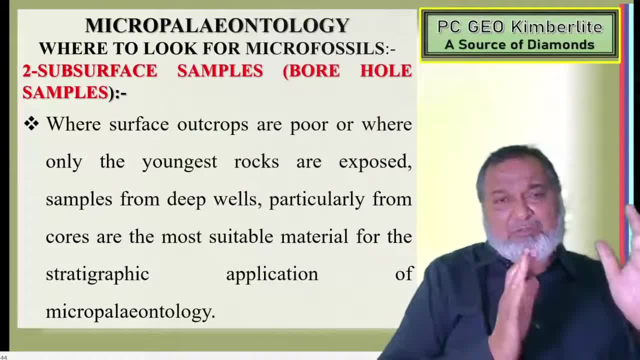 Now the second one: subsurface sample. Now, whatever we have seen, outcrop is done. Now the second one: subsurface of the sample, borehole samples. Here the technique will be required because whatever the sample is there, it is a small one. 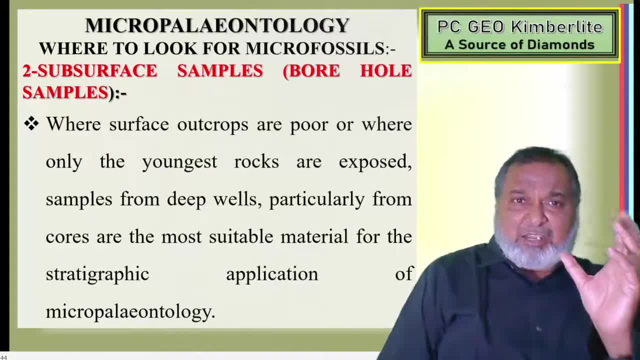 And it is a precious one, because whenever you are taking a drill it is a costly affair, is there? So the sample, small sample, will be given for the research purpose. So from that small sample you have to find out the microfossil. 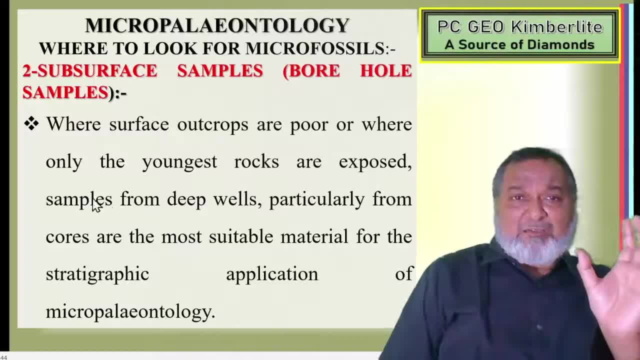 So that is a very, very, very important one. So here, where the surface outcrops are poor or where the only the youngest rocks are exposed, sample from deep wells, particularly from cores, are the most stable material for stratigraphic applications of micropenetralogy. 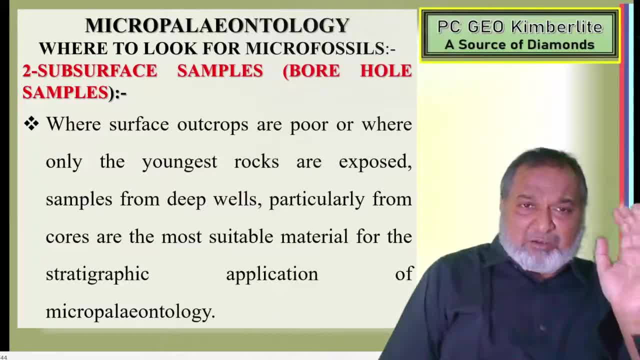 So those who are there in the remote areas, or if you want to take out the sample, from 100 meters, 200 meters, 500 meters, 800 meters, 2 kilometers, 3 kilometers down, So there you have to take the help of the microfossil, because if you want to go for searching the oil and natural gas, 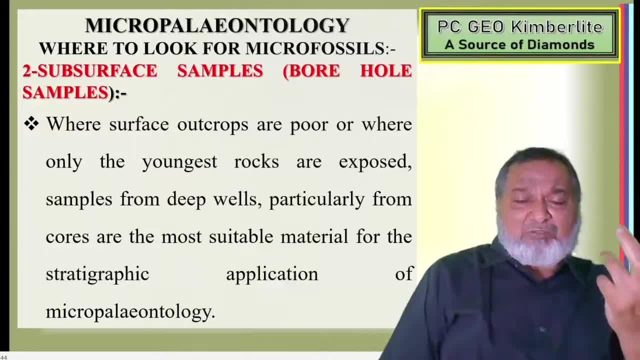 So we have been drilling out the material And we are trying to find out the source rock, that is, the limestone, sandstone, shale mud, And particularly in that we are going to search for the fossils, the polons, spores, poraminifera, astrocots. 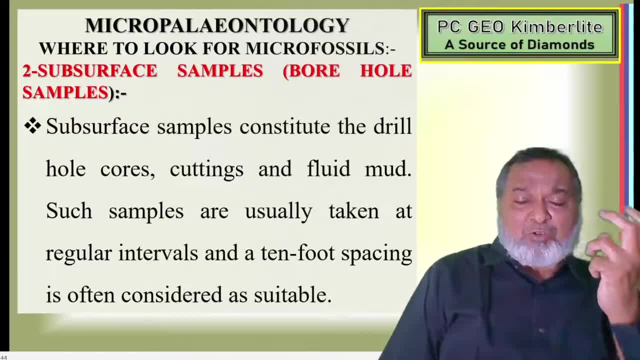 So applications of perimetrology is a very, very important one for the boreholes. The subsurface sample constitute the drill hole cores. cuttings are there and fluid mud is there. Such samples are usually taken at regular intervals And a 10 foot spacing is often considered as a suitable. 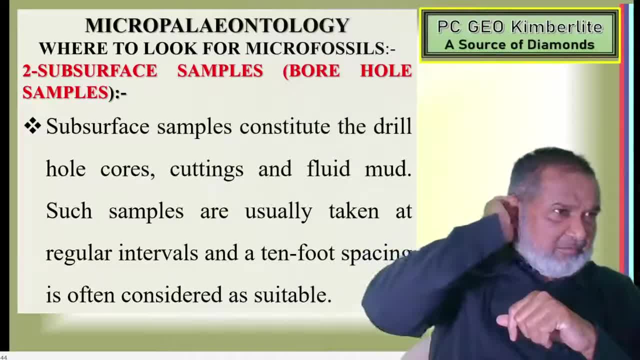 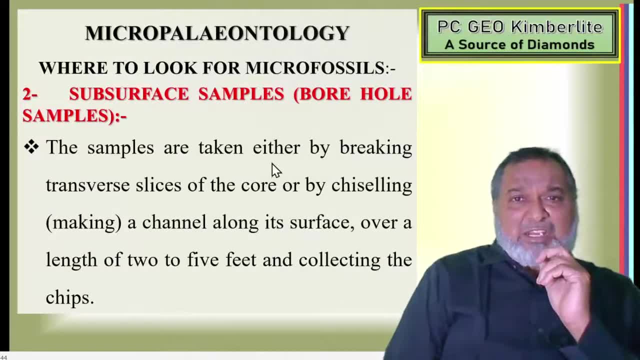 So regular interval of 10 feet? yes, 10 feet will be taken and a sample will be selected and will be analyzed properly. The samples are taken either by breaking transverse slices or of the core or by chiseling a channel along its surface. 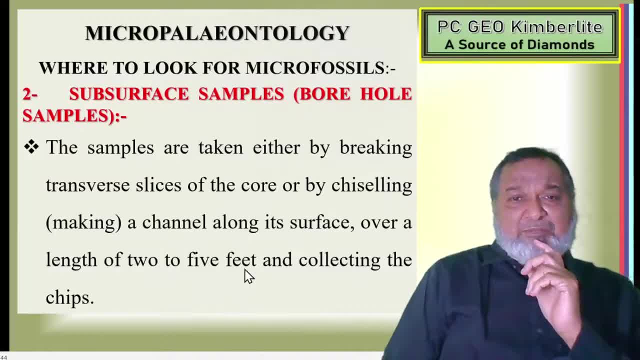 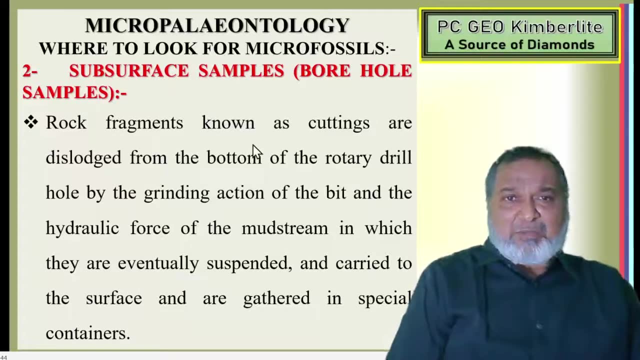 Or Over a length of 2 or 5 feet and collecting the chips. So, vertically or horizontally, we have to take the small, small chips of that particular core sample and we have to go on making the analysis. Rock fragments, known as cuttings, are dislodged from the bottom of the rotary drill hole by grinding action of the bit and the hydraulic force of the mud stream. 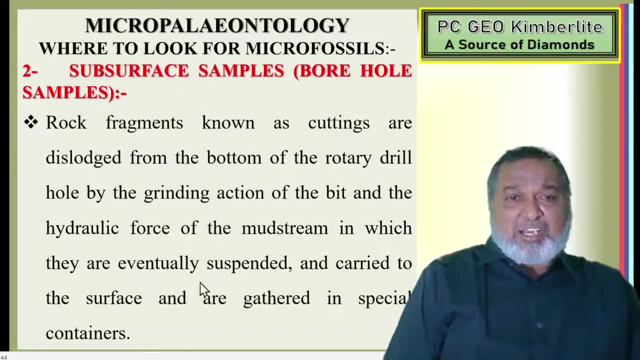 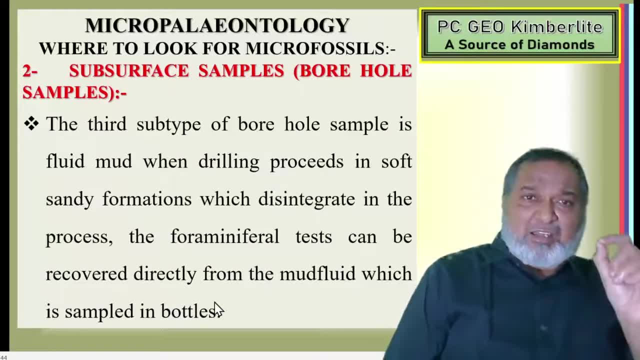 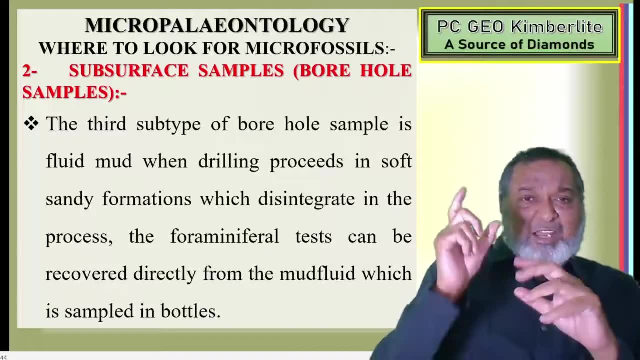 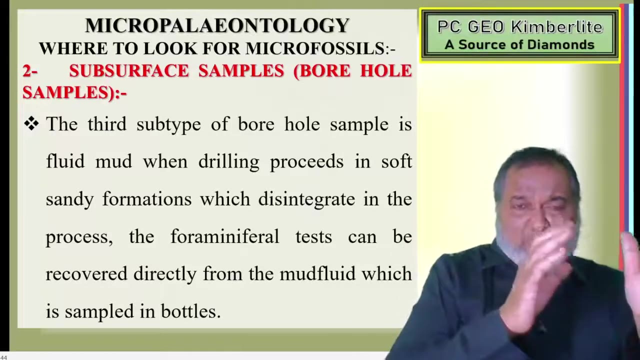 In which they are eventually suspended and carried to the surface and gathered in the special container. Yes, they are kept in a special container and the arrows have been marked So which are the direction. that is, bottom and top has been easily recognized and the depth wise, where what will be the depth is. that has been mentioned properly on the boxes also and on that particular core sample also. 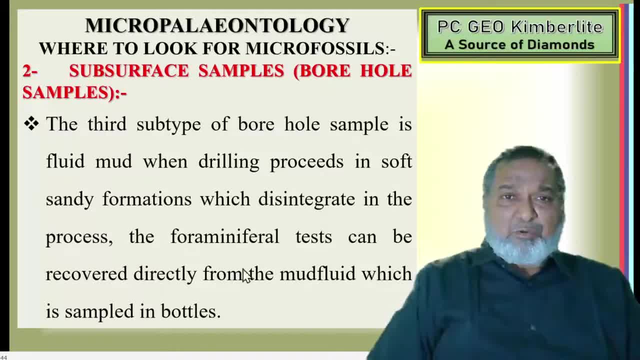 So it has been mentioned so that anything if you want to make out the reference and find out, if you want to make the analysis of that particular core sample, whether it is contained or for micro fossils or not. So the details has been there and with the logs we had to find out, with the regular interval, samples will be collected. 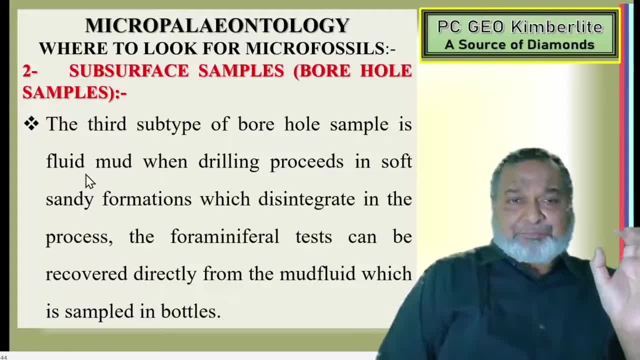 The third subtype of borehole sample is fluid mud When drilling proceeds in the soft sandy formation which is disintegrated in the process, and the foraminifera test can be recovered directly from the mud flow fluid which is sampled in the bottle. 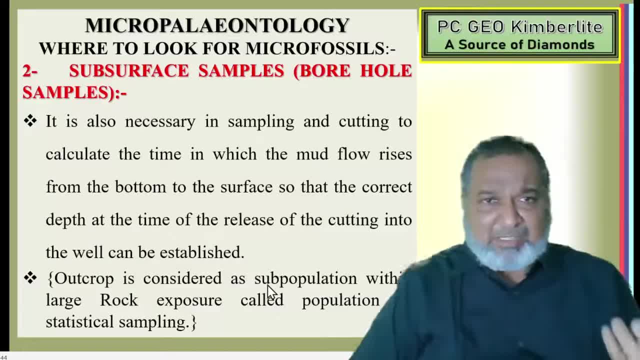 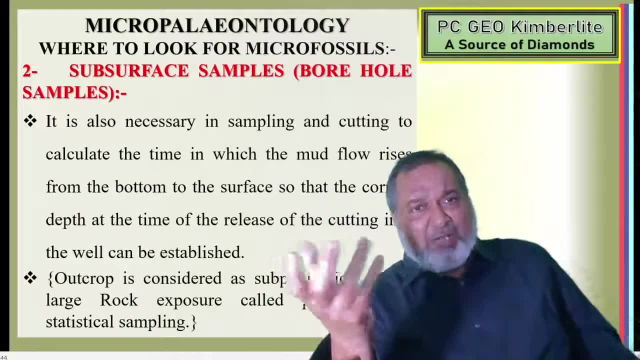 So if the rock is a very soft and fragile is there and drilling is there, then that type time we could not get the core sample. So at that time from that flow, muddy flow, we can separate it out, the micro fossil, and we have to pick it out and put it back. 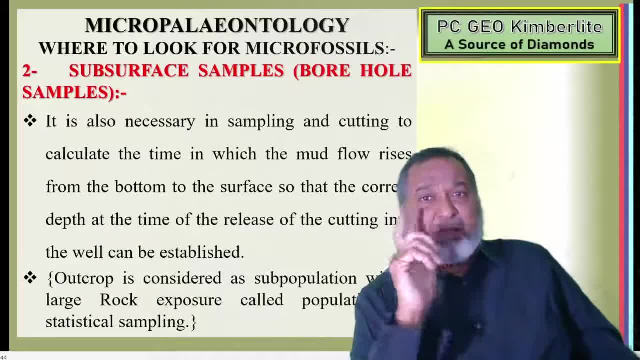 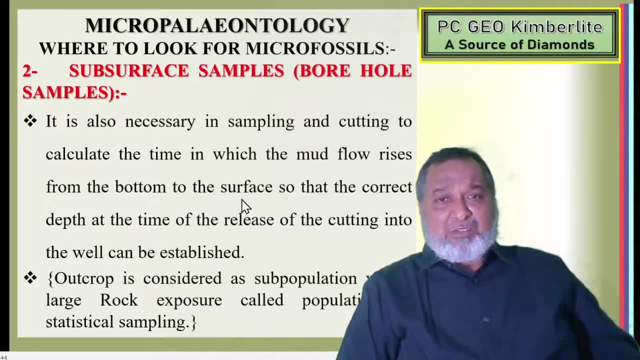 It is necessary in sampling and cutting to calculate the time in which the mud flow rises the bottom to the surface so that the current depth at the time of the release of the cutting into the well can be established. This is the very, very important calculation will be there when it is drilling is taking place. 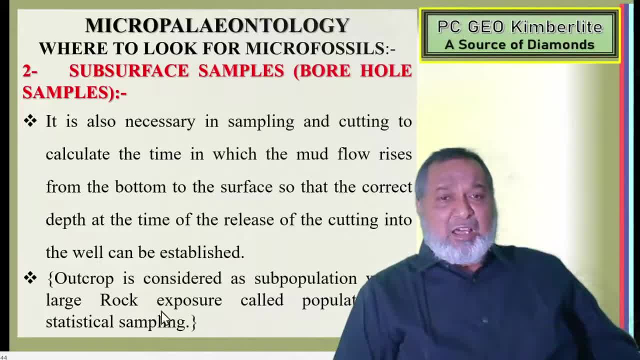 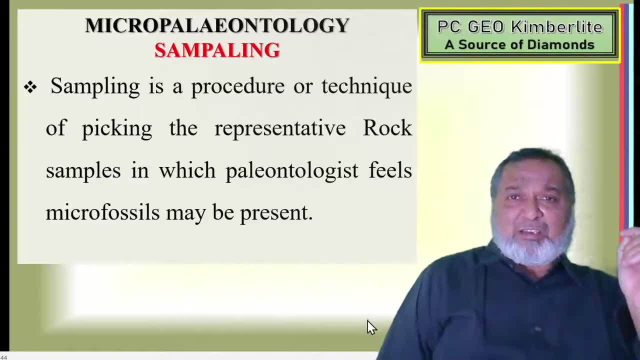 The outcrop is considered as subpopulation within the large rock exposure called population. In the statistical sampling is next one. The title will be the sampling. So how you're going to make out the sampling of microfossils? sampling is a procedure or techniques of picking the representative rock samples in which hydrologist field microfossils may be present. 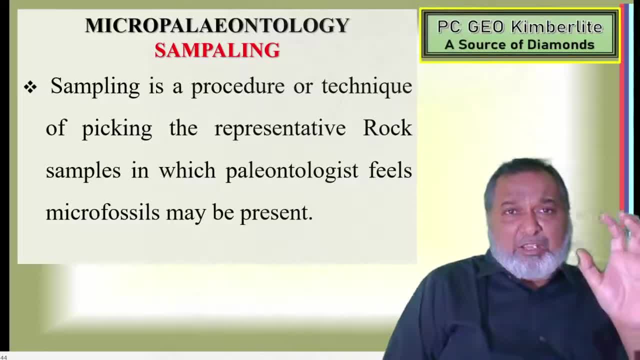 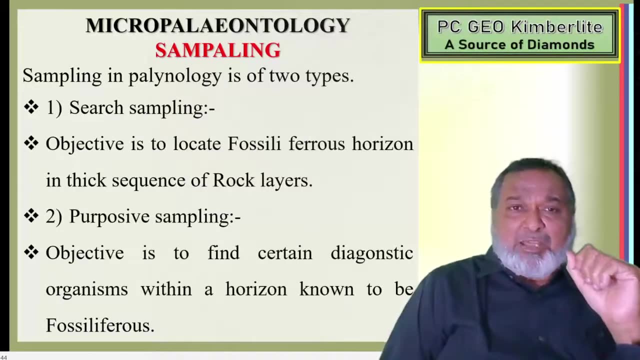 So when you're going to pick out any rock into the sampling techniques, The paleontologist believe that whatever sample I'm picking out in that it should contain the microfossils. So this is what we have. the belief is there of a micro paleontologist sampling for FYBs in our specially 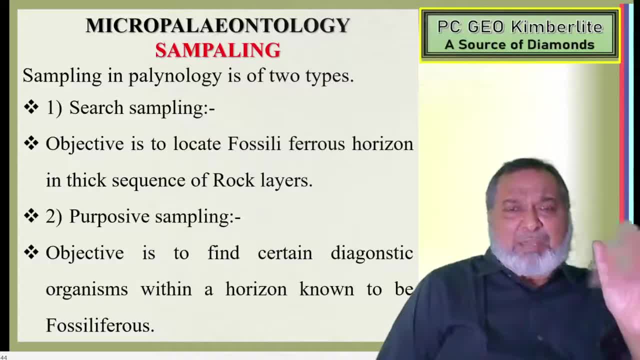 We have only a two sampling techniques are there, but I'm, in addition, I have whatever the sampling techniques are there and just verbally discuss out of sampling in paleontology. So this is what we have. the belief is of two types. So sampling just to go on searching. that is the objective is to locate the fossiliferous, fossil of horizon in thick sequence of the rock layer. 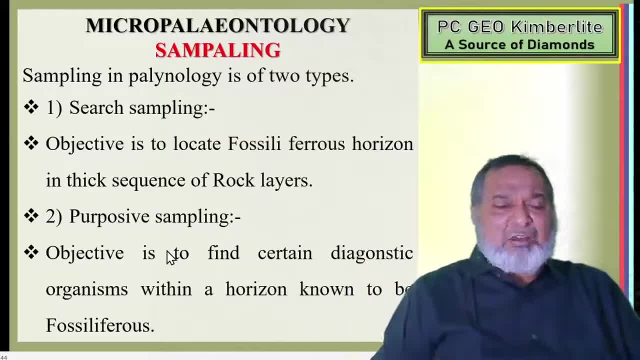 So sampling, just you go on to find out sample, collect it out and put it out. That is the simple. so sampling, purposive sampling, The objective is to find certain diagnostic organism within the horizon known to be fossiliferous. So purpose: Just picking out the micro for a minifera. 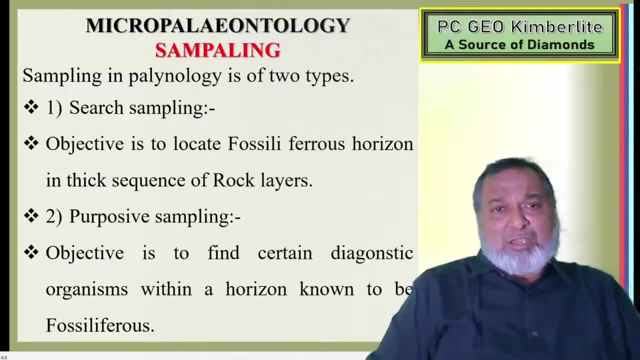 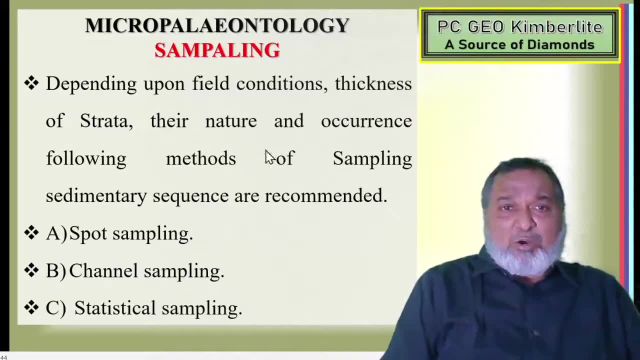 So that is my purpose. is that so purpose sampling. So the purposive sampling that is called as, depending upon the field techniques, thickness of strata and their nature and occurrence, following methods of sampling sedimentary sequence are recommended. Yes, now here, depending upon field conditions, thickness of strata and their nature and occurrence, following methods of sampling in sedimentary sequence are recommended. So the purpose- sampling, just you go on searching, that is the objective- is to locate the fossiliferous fossil of horizon in thick sequence of the rock layer. So sampling, just you go on searching. that is the objective- is to find certain diagnostic organism within the horizon known to be fossiliferous fossil of sedimentary sequence are recommended. 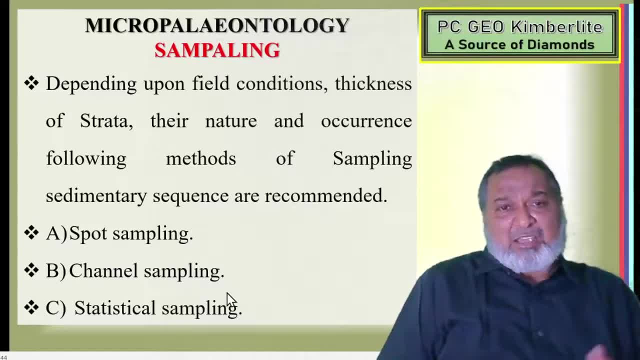 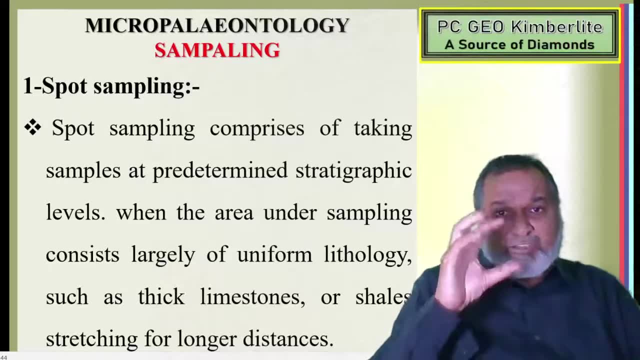 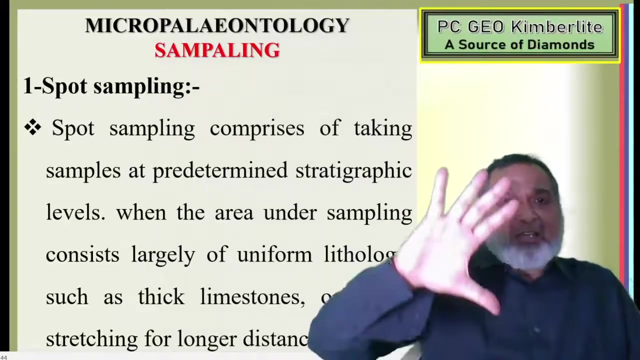 Spot sampling, channel sampling, statistical sampling- these are there in the FIVC so I taken this three. So first one will see the source spot sampling Spot we are going to make out. the source sampling comprises of taking sample at predetermined stratigraphic level. say, I am going to make out that after regular 10 inches I am going to take a sample, or after a regular 1 feet I am going to collect a 1 sample. 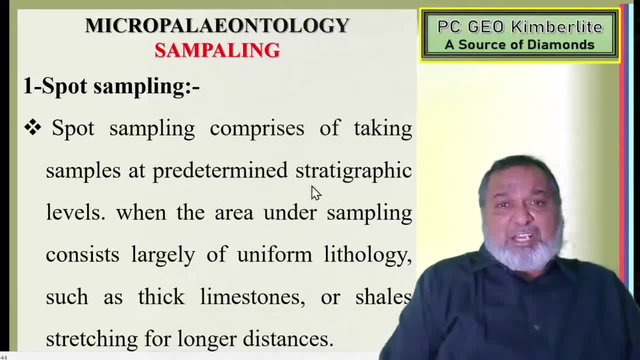 So that is my spot sampling, my spot sampling when predetermined stratigraphic level, when the area is under sampling, consists largely uniform lithology. when you are going to make out this one, when the, whatever the bed which is exposed in that area, it is a large one, say it may be a meter together or it may be 10 feet. 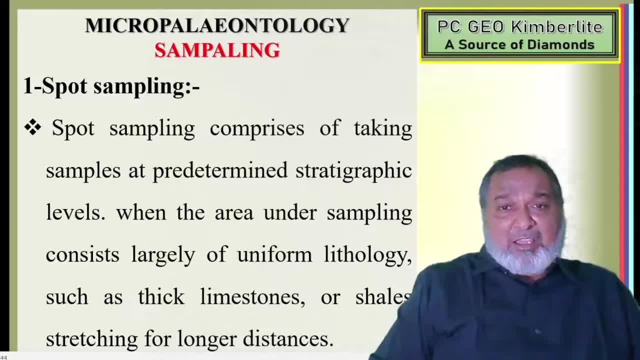 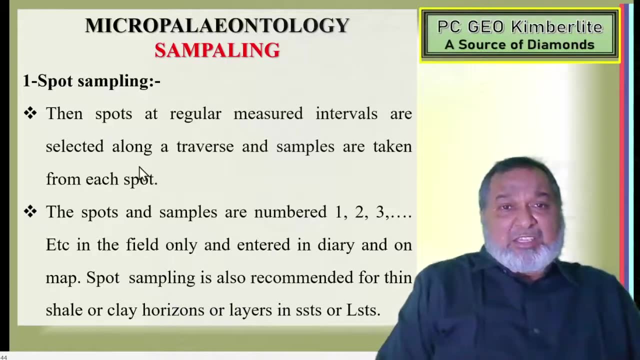 solid. so that will be there. so in that we can make out that particular, yes, so largely uniform lithology such thickness, thick limestone or shell stretching for a longer distance, for this we are using the spot sampling, then spots at regular measured interval are selected along the transverse. 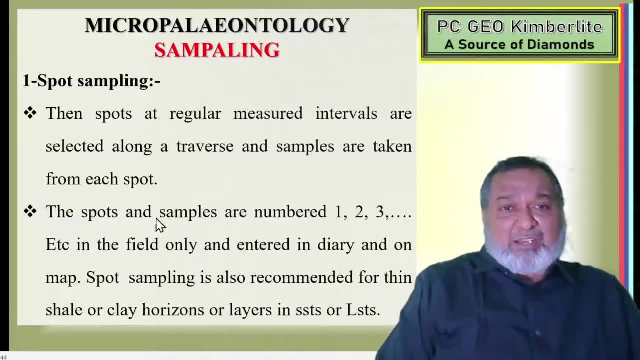 and samples are from each spot will be collected. the swat samples are numbered one, two, three, etc. like this in the field only, and enter in the variety and on the map. spot sampling is also recommended for thin shells, clay horizons or layer in sandstone and lampstone wherever thin material is there. so 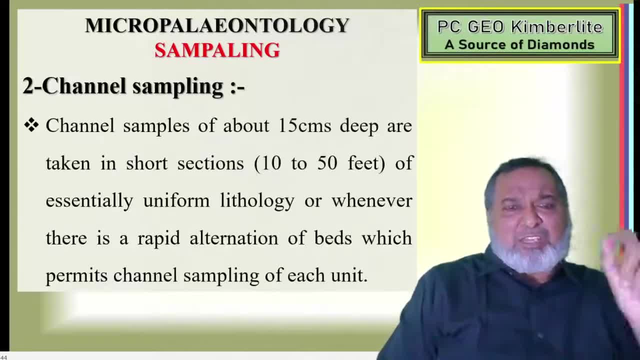 which are any forming thicknesses are there. so in that also the thickness will make out regularly and we can find out the, whatever the distance will be there where it will be less one second. one channel sampling- channel sampling is about 15 centimeter deep- are taken into short section. 10 to 50 feet are essentially uniform lithology or wherever. 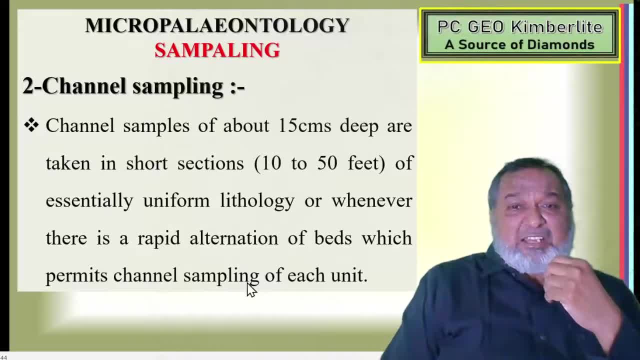 there is a rapid alteration of bed which permits channel sampling of each unit. so from the 15 meter deep are taken in short section of 10 to 50 meters of essentially uniform lithology. and wherever there is a rapid alteration of beds are there which permit channel sampling of huge. each unit small. 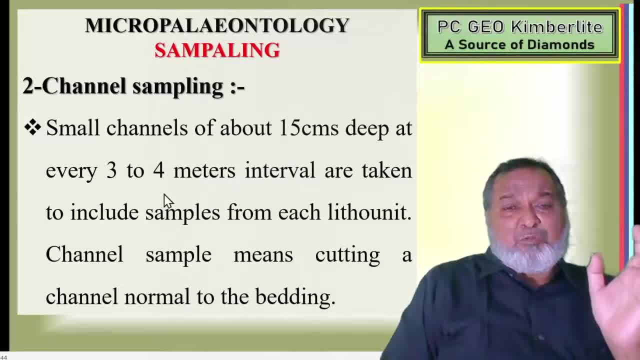 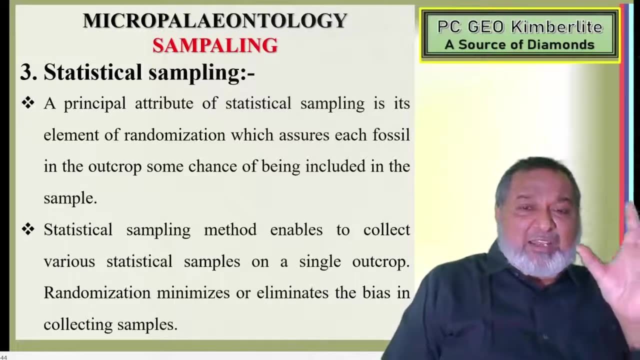 channels of 50 centimeter deep are at three to four meters interval, are taken and include sample from each litho unit. Channel sample means cutting a channel, normal to the bedding, Next one statistical. So here we have. number has been fixed, A principal attribute to the 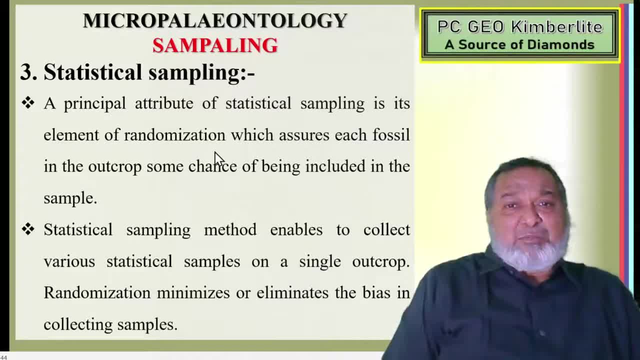 statistic sampling in its element of randomization, which assure that each fossil in the outcrop some chances of being included in the sample. So 100 sample, 200 sample. So whatever the sampling, we assume that in that area good sample, we can collect it out. So we fix the number I want. 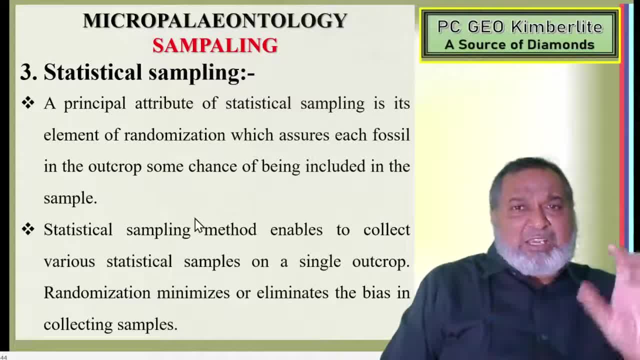 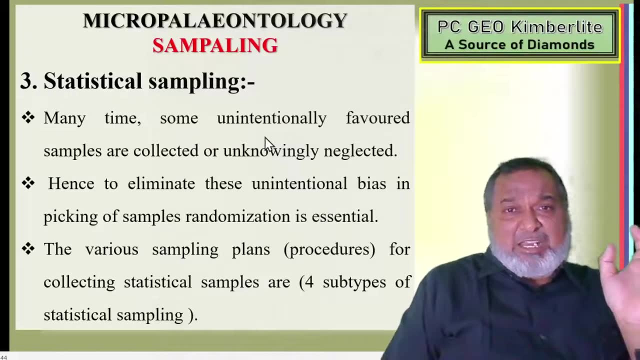 10 numbers of fossils, I want 5 numbers or 20 numbers. So on that we are okay. Statistical sampling method enable to collect various statistical sample in a single outcrop. Randomization minimizes or eliminate the bias in the collecting samples. Many times some. 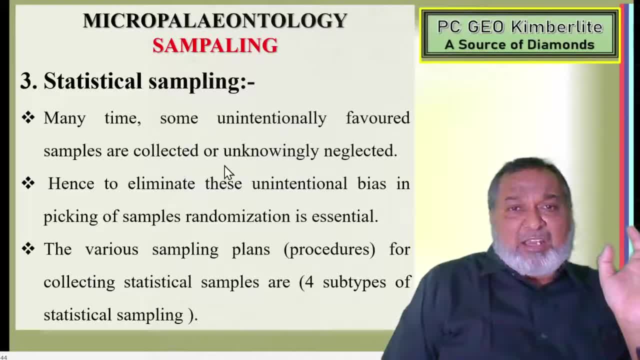 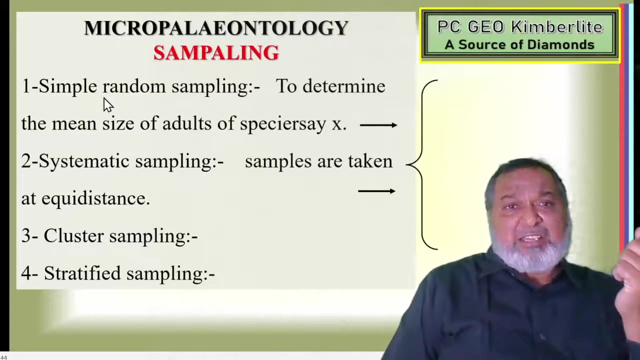 unintentionally flavored samples are collected and unwillingly neglected. Hence to eliminate these unintentional bias in picking the samples in randomization is essential. The various sampling plans, procedure for collecting statistical sampling, are the four subtypes of the statistical sampling. In this statistical sampling, one is simple random sampling to determine the 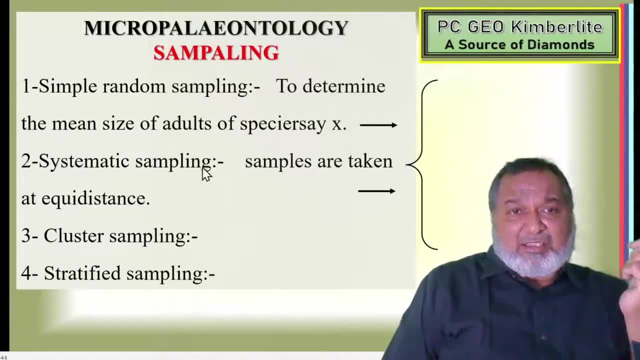 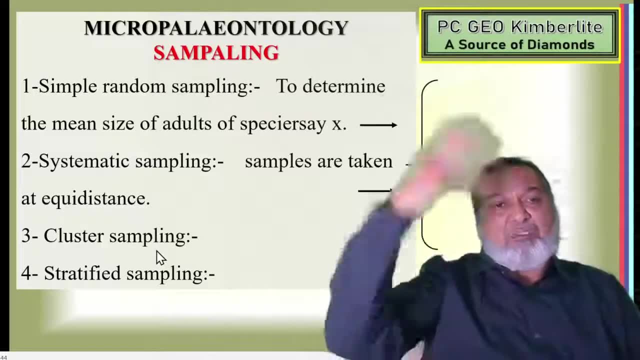 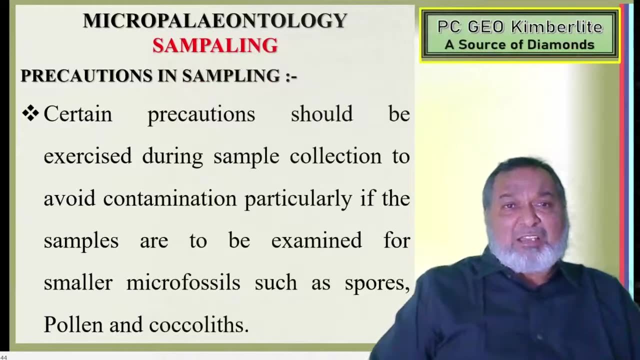 mean size of the adversities, where spaces, say x, Systematic sampling sample are taken at equidistance. So the sampling is simple: We are going to make a cluster and from that we are going to pick out Stratified sampling. From the east stratified bed we are going to collect the sample. So these are the 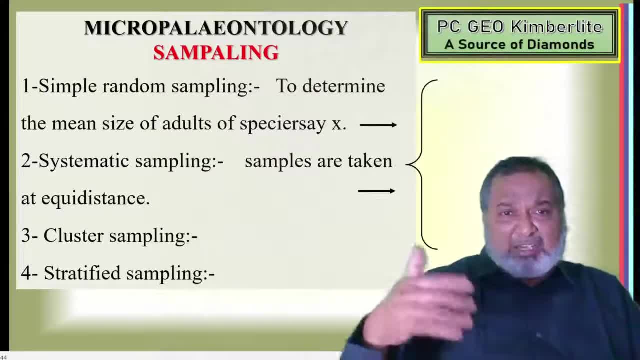 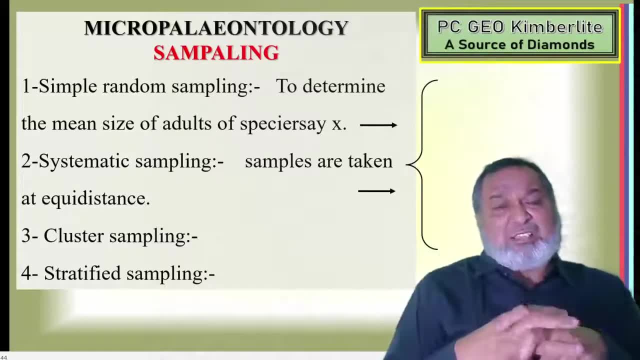 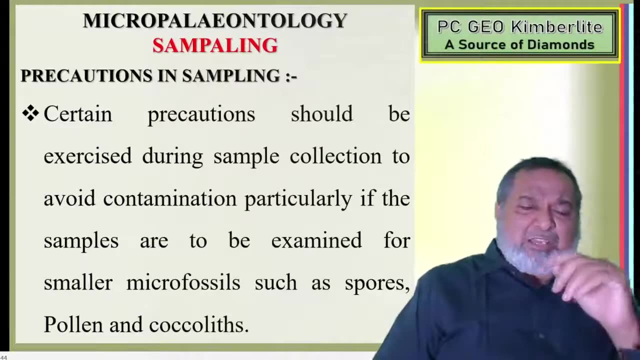 various part which have been making out In addition to this one: stratigraphic sampling, search sampling, spot sampling, channel sampling. So these are the sampling is there, but in the examination only the spot sampling, channel sampling. these are the thing which we will ask, But statistical sampling. 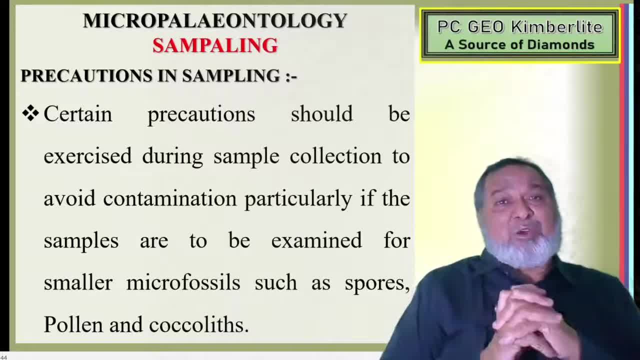 nobody is going to ask you. Now the next one in this: the precaution in the sampling. What precaution you have to see taken into the consideration when you are going to collect the sample? Certain precaution should be exercise during the sample collection to avoid contamination. That is a very, very important When you are going to collect the sample there. 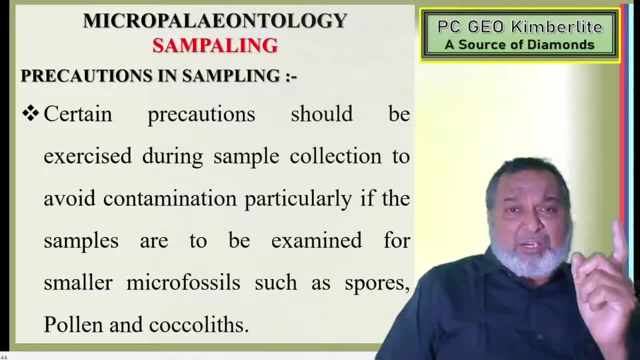 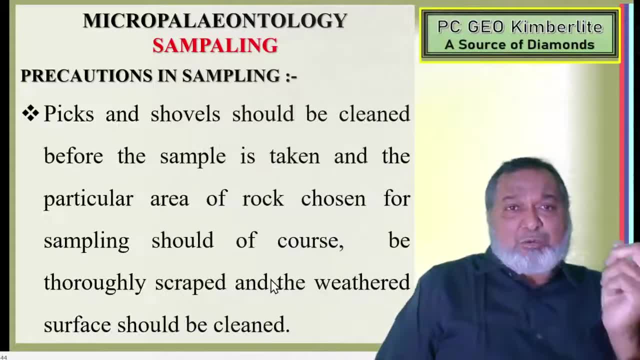 should not be any contamination. You have to take very care, particularly if the samples are to be examined for a smaller microfossils such as spores, pollens, cocolate Picks and shovels should be clear, clean, before the sample is taken. Everything has to be clean, Say, once you are used next time. 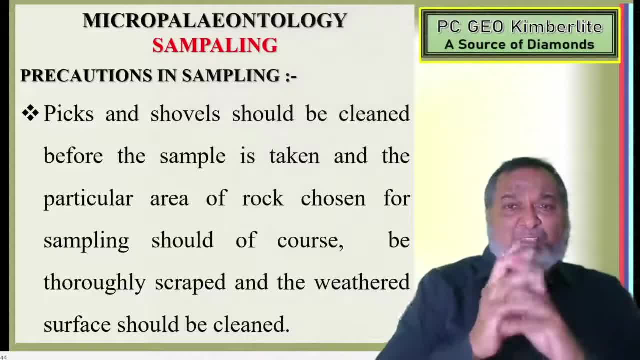 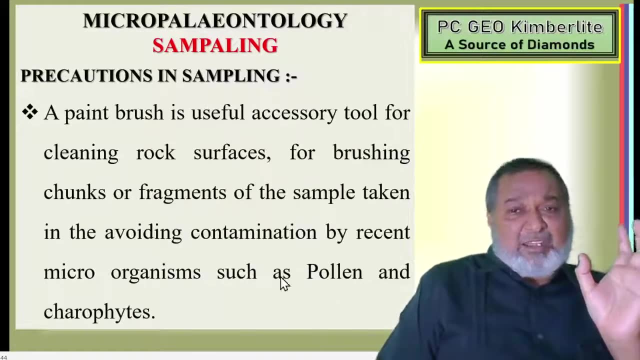 you have to clean and then only you have to go for picking the sample with the shovels. Particular area of rock chosen for sampling should be, of course should be coarse, not of course coarse, and between Generally scrap, the weathered surface should be clean. Yes, you have to keep all into the mind that. 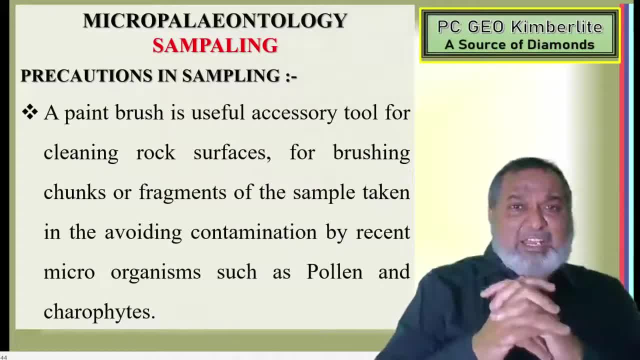 whenever you are going to take a sample, it should be from a clean and fresh sample. So from fresh rock sample you have to collect the sample- Very important one. Then you are going to use the brush. pen brush is usually accessory tool for cleaning the rock surface, For brushing chunks and fragments. of sample taken in avoiding Contamination. So there are number of fibers will be there, hairs are there. So when you are going to clean out the surface, see that next time when you are going to use out, clean thoroughly that brush so that anything should not be there. Otherwise, if any fossils, pollens or spores are there, then it will be contaminated. So don't have to make very precaution as to it. Make out when you are taking a use of it. 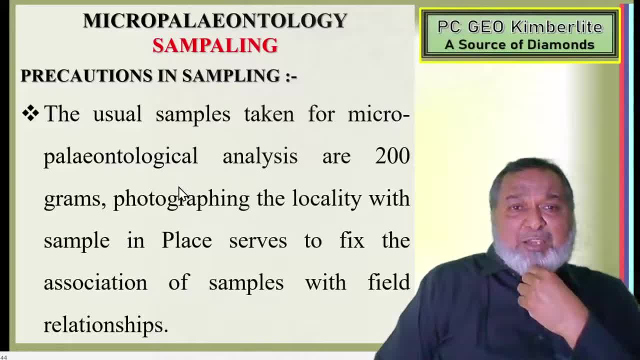 Using the brush. the usual sample taken into the micro chemical analysis are two hundred grams. Yes, the usual sample taken for micro chemical analysis are 200 gram. Photogramming- the locality with the sampling plays serves to fix the association of the samples with the field relation. so, keeping into the view that if 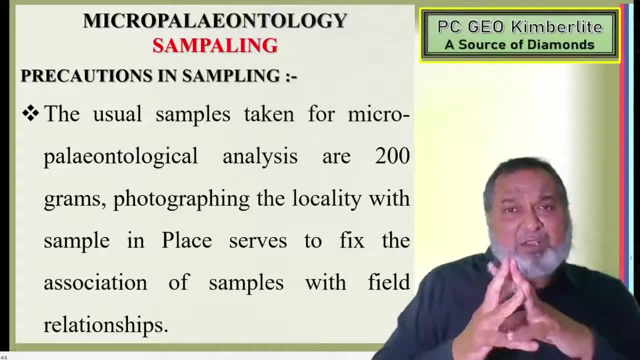 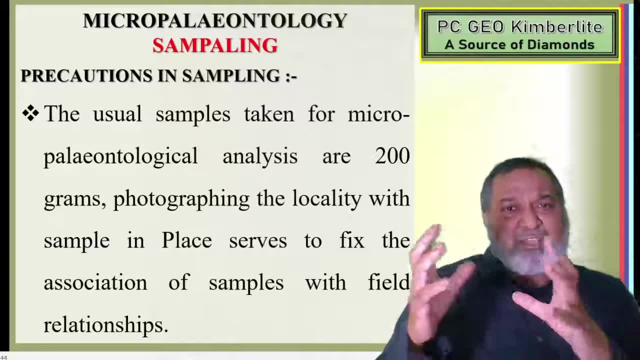 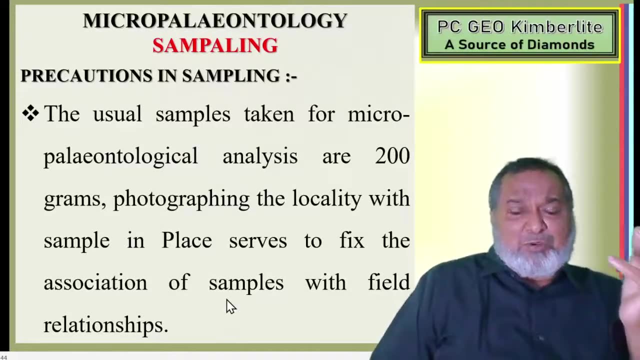 we require the micro pathological analysis, a sample will be require then. it should be at least 200 gram, But keeping in that we are going to use several times, then instead of this directly, you can take out one kg sample. so that has to be carried properly. so how much material you have to carry properly till to fill to the your area. 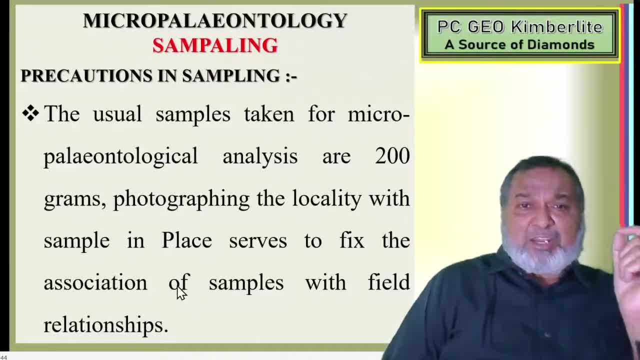 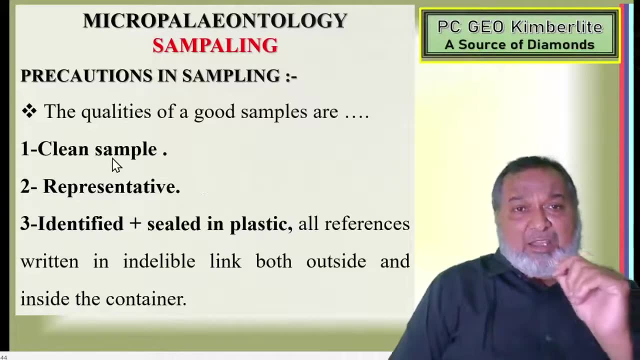 destination. so keep into the mind and you have to take properly the weight of the sample and the locality of sample in place supposed to fix and associate sample with the field sampling, with caution in sampling. yes, the qualities of a good samples are a clean sample, representative identified and ceiling plastic. once you get the clean sample, represent that you identified and 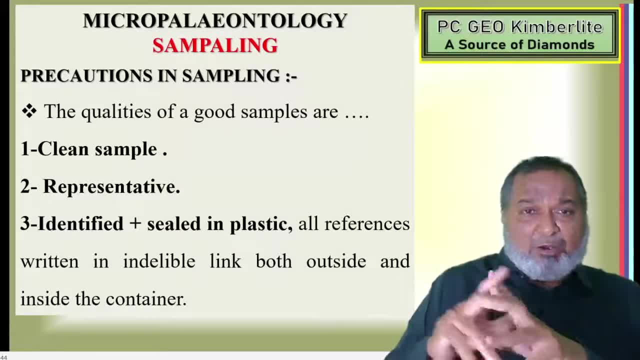 now it has to be sealed in a plastic, all has to be done. and yet we written in in the indigable, in both outside and inside the condor, sometime in the plastic bottle as well as the plastic bottle, as well as in the plastic bottle, as well as in the plastic bottle as well. 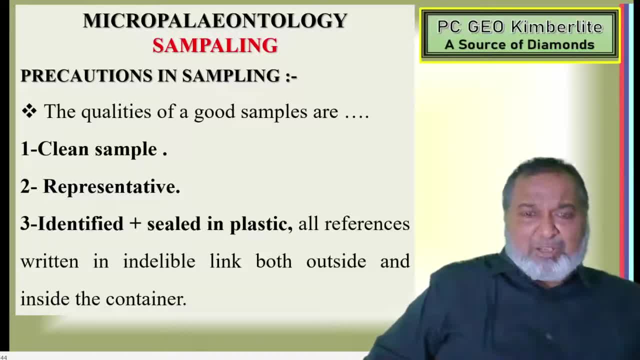 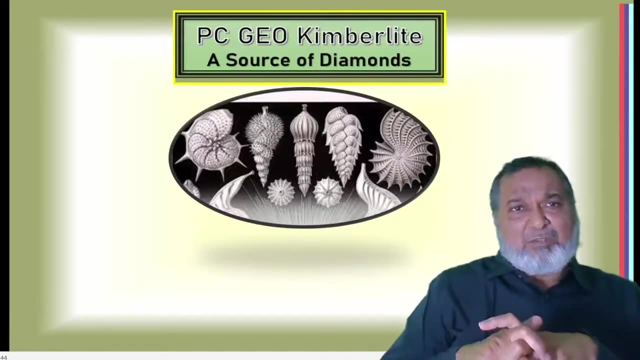 as your plastic polythene bag also put down the whatever you are writing, the points are there. you have to write down and put it over there and on the surface also you have to mention the thing, that, what it is there in that container. I think this will be clear today that whatever we have, the techniques are there, the spot. 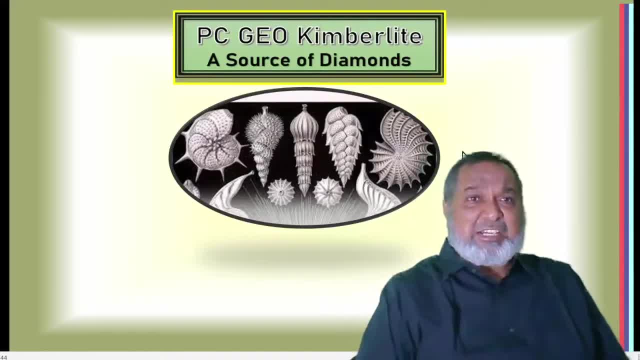 sampling, channel sampling, statistical sampling and the statistical sampling. So these are the normal samplings, are there so, which we are going to use in the microfossils. but whatever the you are going for a collection of microfossils, patient should be there and 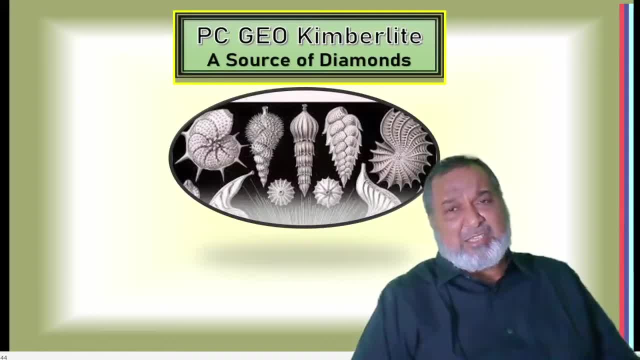 whatever the delicacy is there, cleanliness is there? proper handling should not be contaminated. that things, once you are taken into the consideration, then there will be. once you are done all these field work and collect the sample properly, Come into the lab and keep the samples at a proper place and, one by one, you have to.